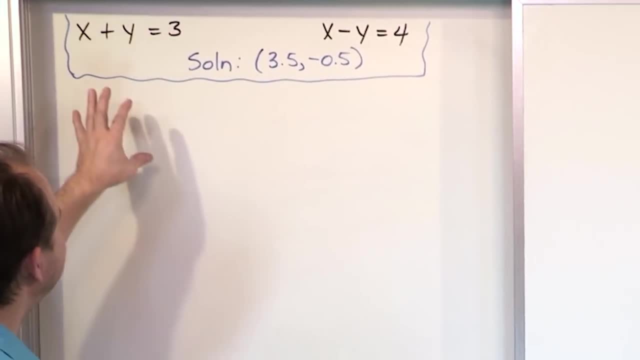 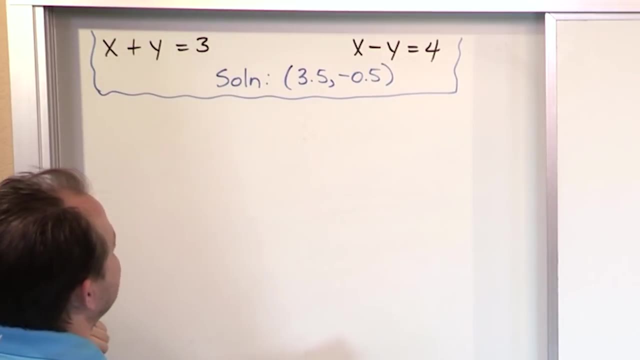 an exact way to do it. So what we have on the board is the very last problem we solved in the last section. I gave you this equation. I gave you this equation. We put them in a slope intercept form, We graph them And from the graph we figured out that this is 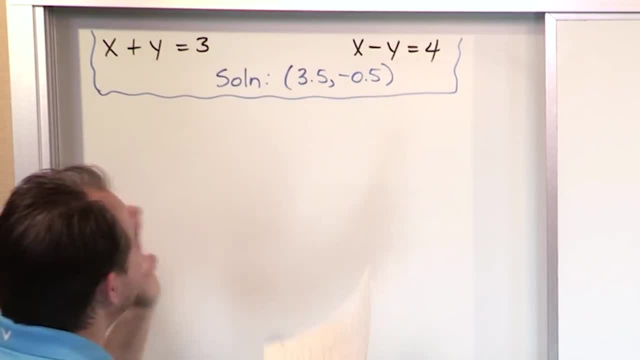 the solution: X is 3.5 and Y is negative 0.5.. So this is an equation that we've already solved And we're going to do this a lot. We're going to be solving a lot of these problems. 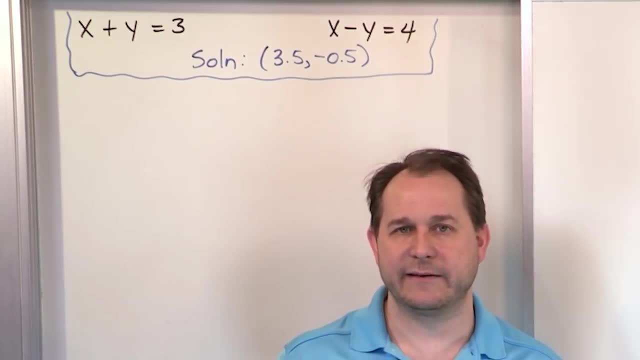 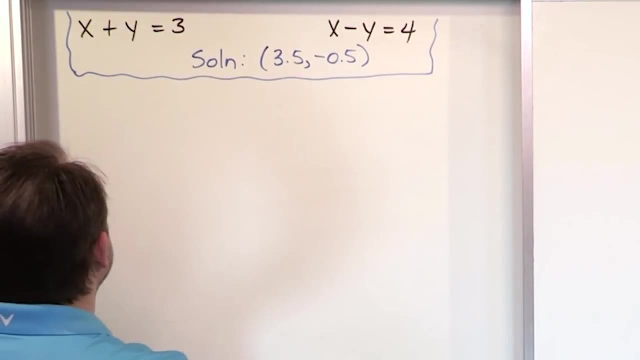 We've already solved them by graphing. We'll be doing them just a different way to get the same exact answer. so we can kind of verify, you know, that the answers are correct. So here's what we're going to do. Let's take the first equation And just I need to get. 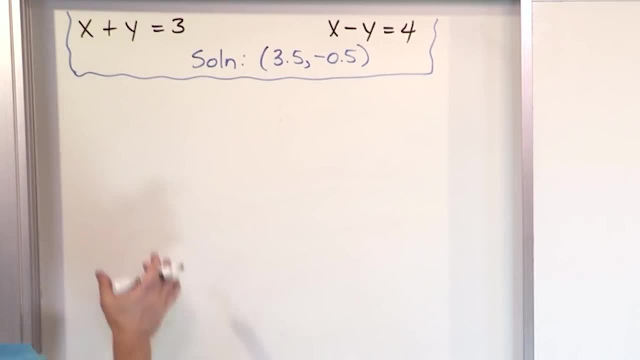 through a couple of problems for you to get the hang of it. So for now, just kind of go with me. Let me take the first equation and let me solve for Y, just like we've done many times before, I'll say that Y is equal to negative X plus 3.. How do we get that? Because 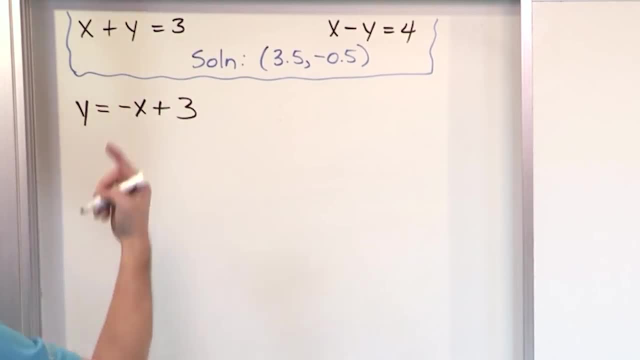 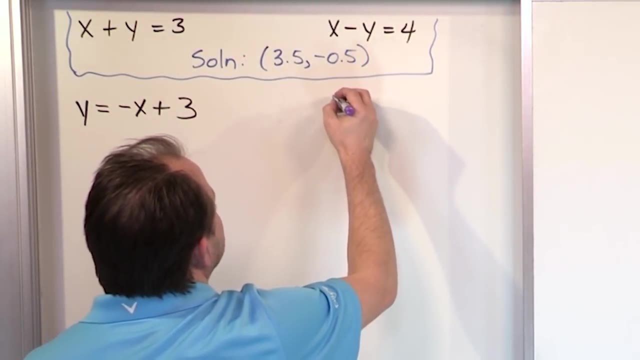 we subtract X from the left, we subtract X from the right. So we just moved it around and we made it equal to this. Now, this equation over here, I'll switch colors. I'll do the same thing. by solving for Y, I will say: negative Y is equal to negative X plus 4, right by. 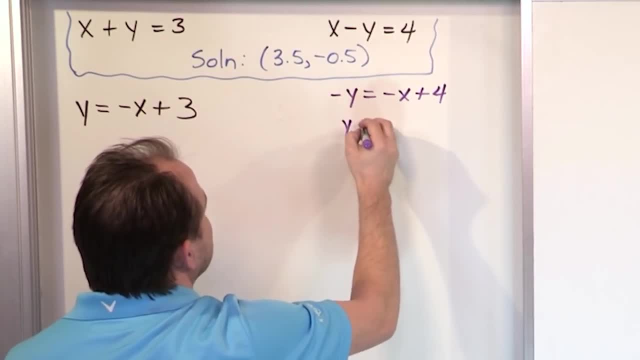 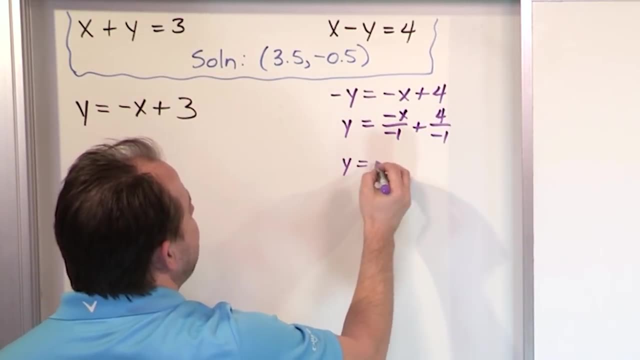 just subtracting X from both sides. Now we have to divide by negative 1.. So it'll be negative X over negative 1, plus 4 over negative 1.. So here we have a division, We'll have X And here we have the minus sign. that's. 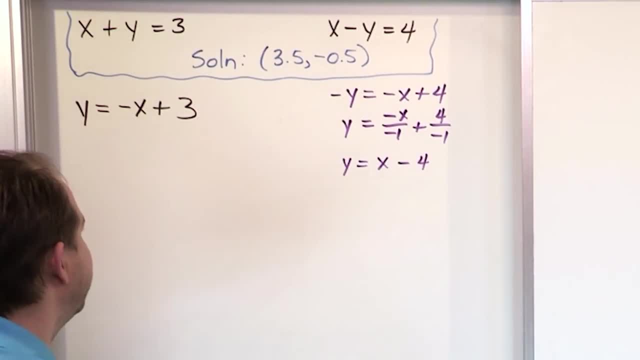 going to float up and it's going to make it minus 4.. So we have X minus 4 over here. So in this case I'm giving you these two equations, But I could have also in a separate problem. I could have just given you these equations And I'm going to ask you the question Solve. 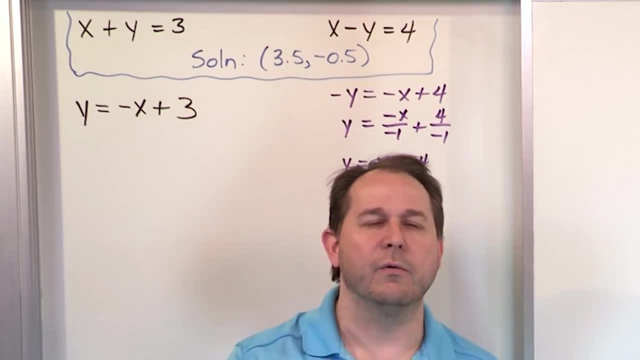 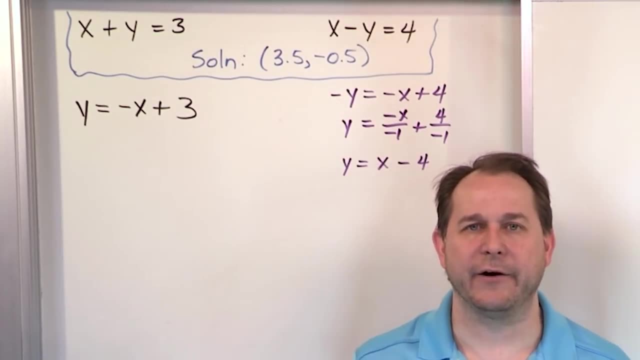 the system of equations, Which means in your mind you know that that means I'm looking for an intersection point that's common to both. In other words, I want to find the XY value, the XY pair, that works if I substitute it. 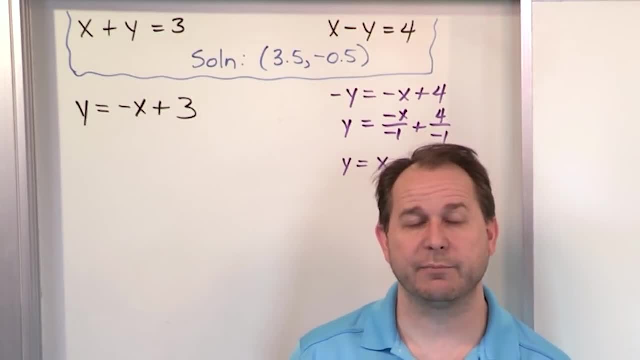 into line number 1, but also works if I substitute it into line number 2.. That's what we've said all along. Now notice what I'm saying here. I'm saying that the Y values of this line is equal to this junk. And I'm saying the Y values of this line is equal to this junk. 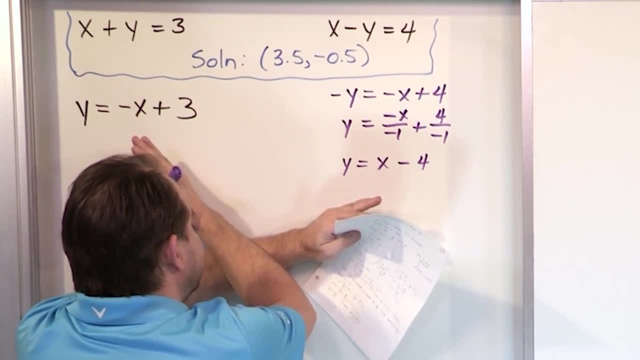 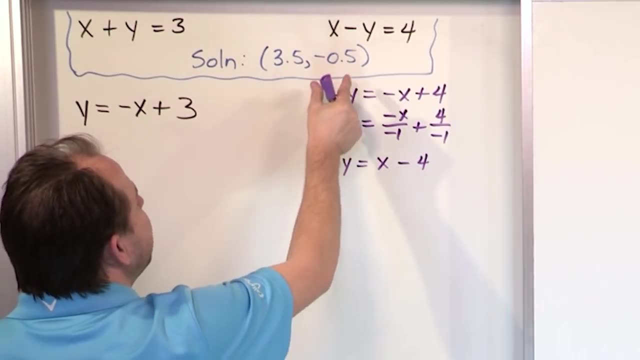 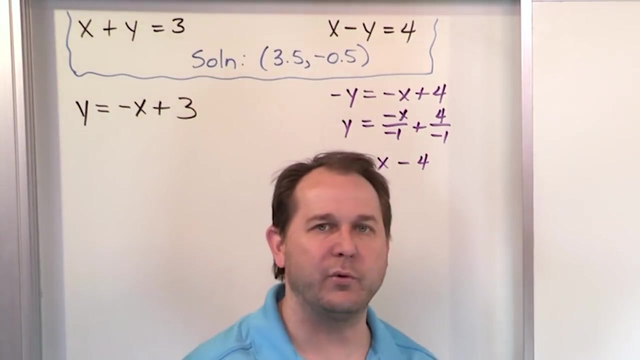 So if there is a point where they cross like this, then it must be true that the because we know that this is the answer right. So we know that the Y values of both of these lines at this point is the same, Because that's what an intersection point is. We intersect. 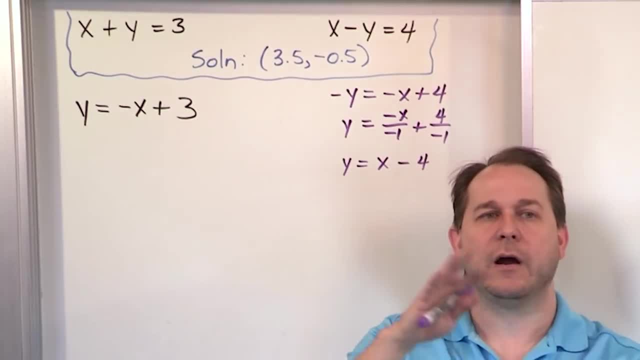 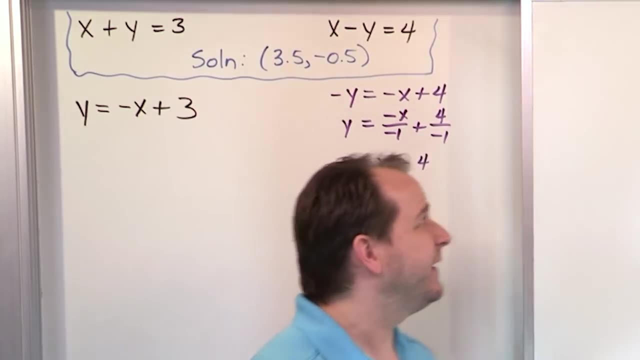 them and we're saying: hey, there's a point here, X comma Y that works for both lines. So if there is a solution to this- which we're assuming there is- then this Y value, whatever it is- I'm pretending I don't know what it is, but we actually do know what it is in. 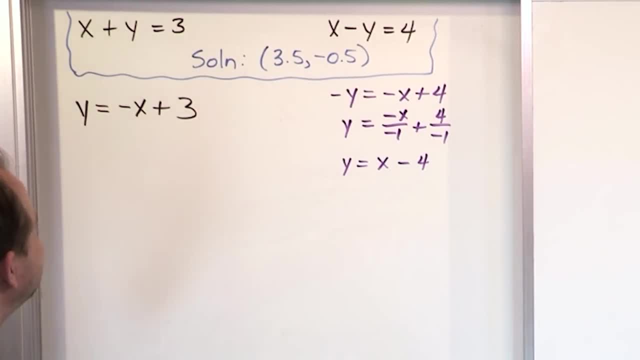 this case has to be the same for both of them, Because the Y values of only thesechi are equal to this and none are equal to they. I can eventually substitute with this line that typically works, the Lie equation: you know, y. So if you're saying that this line is Y is equal to this junk, and we're saying: 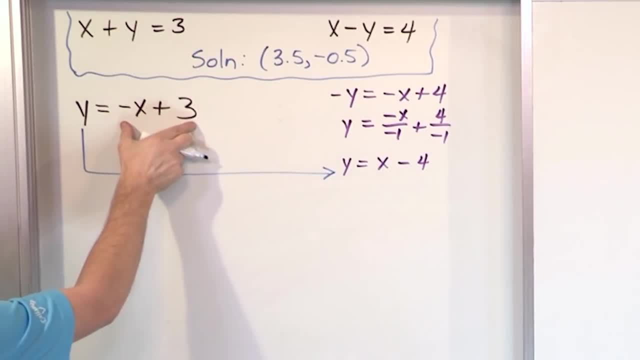 that this line is Y equal to this junk. if there is a solution, then that means I can take this Y and I can plug it into this, Because I'm saying Y is equal to this And here I'm saying Y is equal to this. Well, if I'm saying that there is an intersection point, then 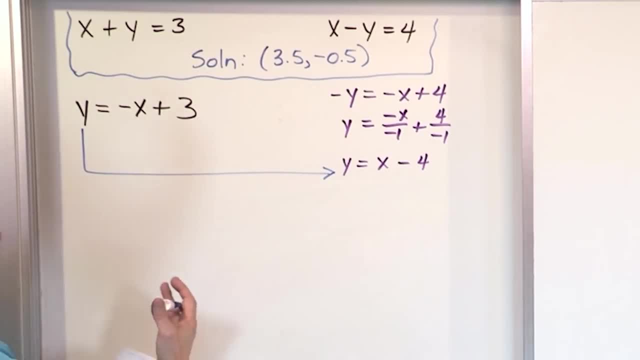 they have to be. I have to be able to substitute what this Y is equal to into this equation. values have to be the same at the intersection point. I'm trying to emphasize that right. So, because you don't know what it is, but you know what. 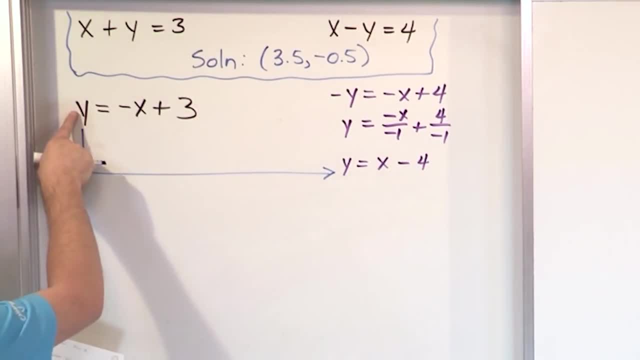 they, they have to have a common y value. So I'm going to take this y value from this equation and I'm going to stick it in here, But I know that this y value is actually equal to this. So I can take this, what it's equal to, and I can stick. 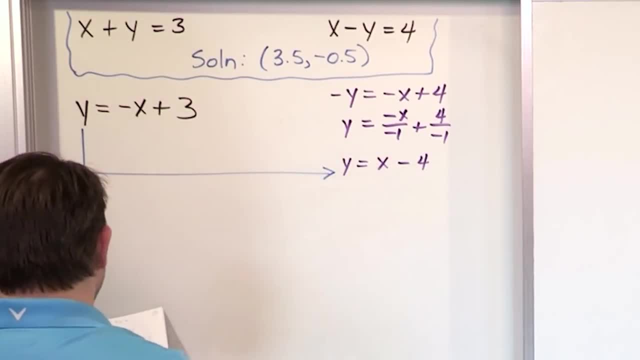 it in there. So what am I going to get? Well, I'm going to get the following. I'm going to say: oh, I'm going to work over here. this is what y is equal to negative x plus 3.. But it's got to be equal to this x minus 4.. It is absolutely. 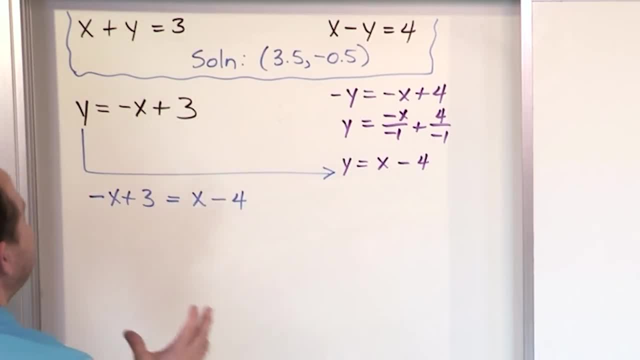 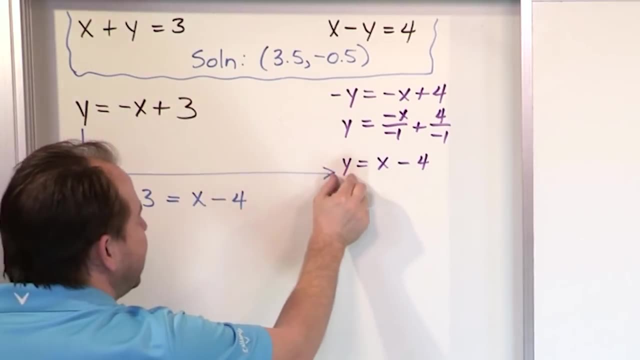 crucial that you understand why I'm doing this. It's because I'm saying there's a common intersection point here. so wherever they cross, the y values have to be the same. So I can substitute y into here, just like any variable can be substituted in right. But I know what y is equal to. It's equal to this, this: 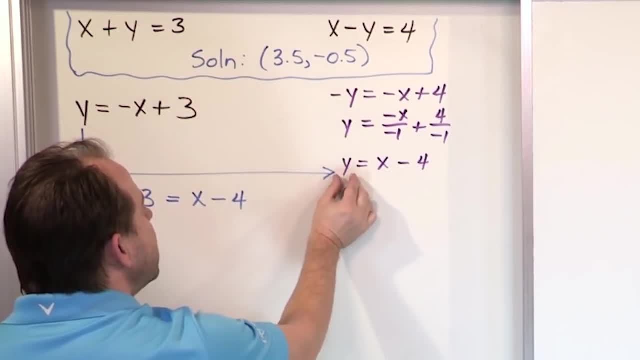 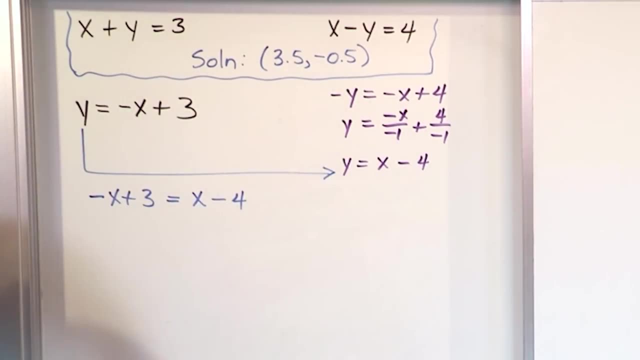 expression for x. So I'm just putting it on the left hand side of the equal sign, because that's where y is. So I just literally stick it in for y right here, just as it sits x minus 4 on the right, this stuff on the left, And then the magic can happen. I can now solve for 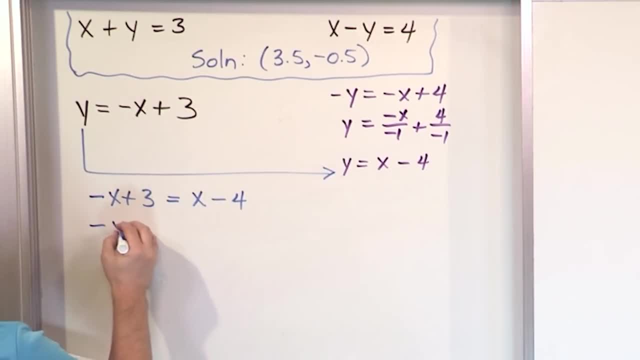 x right, I'm going to move x to the left, So I'm going to have negative x minus x plus 3 is equal to negative 4.. I just subtracted x from the right, subtracted x from the left, which becomes negative. 2x plus 3 is equal to negative 4.. Now I 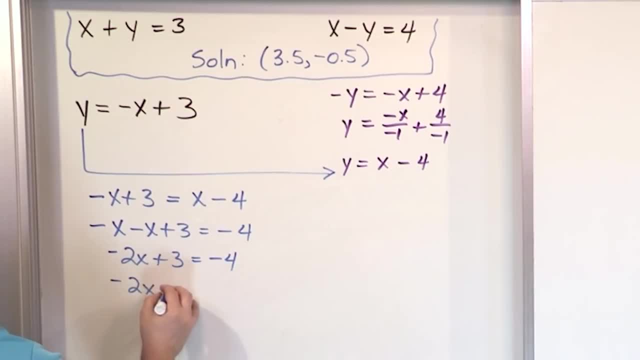 have to solve for x. so I'm going to move 3 to the other side. Negative 2x equals I'm going to subtract 3.. So what is negative? 4 minus 3? negative 7? And then finally to get x by itself. 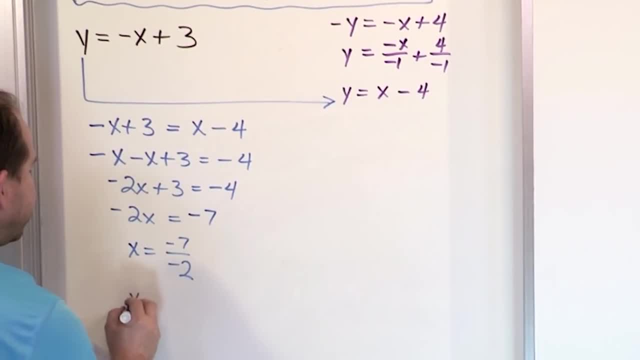 it's just going to be negative 7 over negative 2.. So then x is going to be the positive. it makes it positive. I can't really do this division without introducing a decimal, so I'm just going to leave it at 7 halves. So I'm saying: 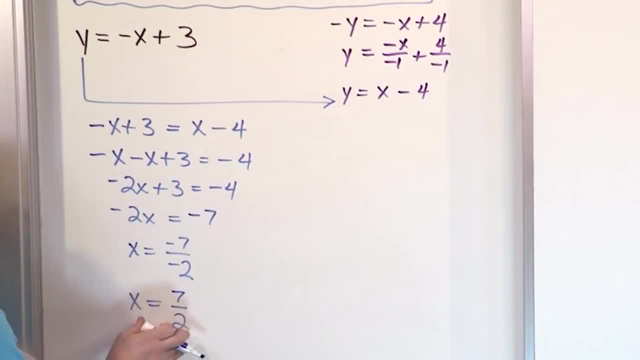 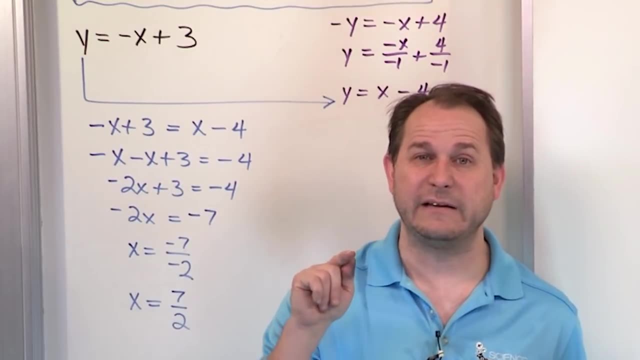 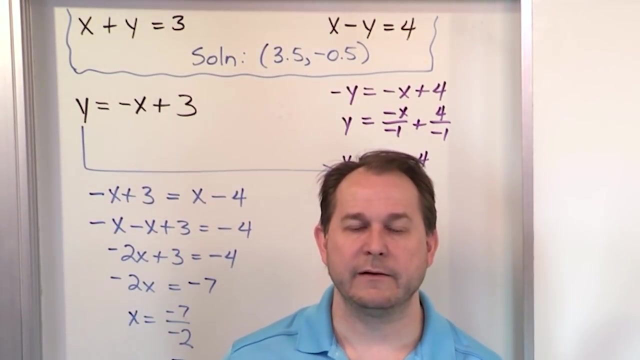 the x value of the intersection point of these graphs is 7 halves, Seven halves, seven halves. If you get a calculator out and you put seven divided by two, what are you going to get? Three point five. What we found- because we haven't found the whole solution yet, but we found that these 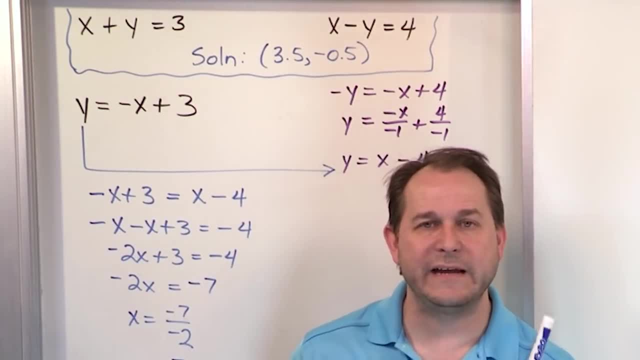 lines intersect in a place where the x value of the intersection point is seven halves, which is three and a half, three point five. All right, so now we have half the answer. This is half the answer. How do we find the other half the answer? 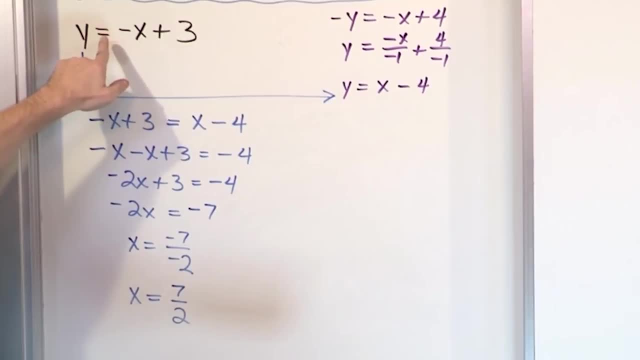 Well, look at what we were given. We have two equations. One of them is: y is equal to negative x plus three. The other equation is: y is equal to x minus four. And now we're saying that we know what the x value is. 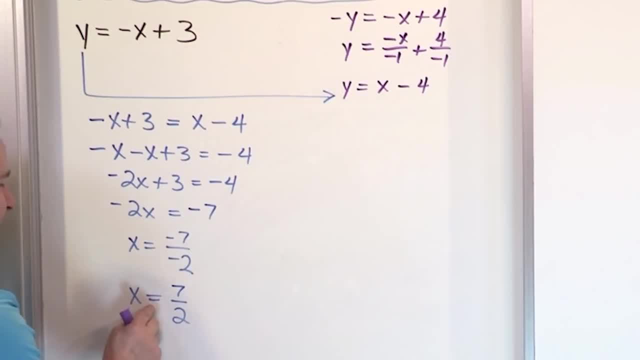 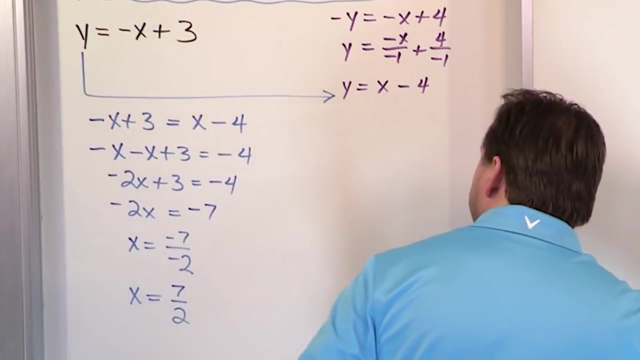 That's the solution of this guy. So if we know this, we should be able to stick this value into this equation, or we can stick it into this equation. Either way we should get the corresponding value of y that works. So let's take this, and I'm going to try to do it with little lines to help you. 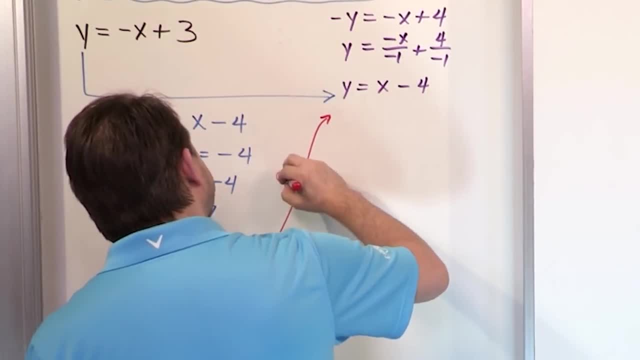 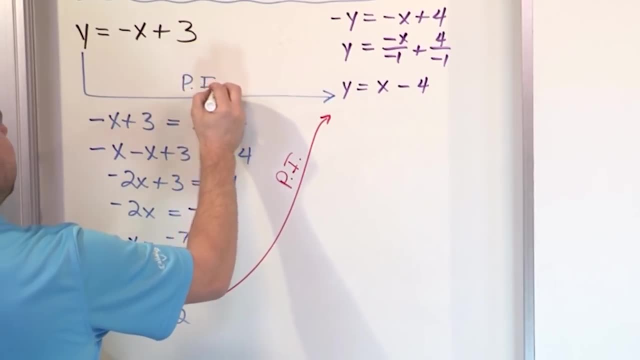 So I'm going to go ahead and say here: when you see me write something like pi, that means plug in, right, I should have written it here also: pi, That means plug in for y. This means plug in for x, right. 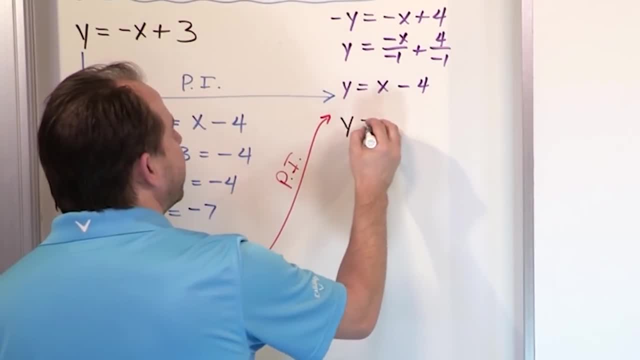 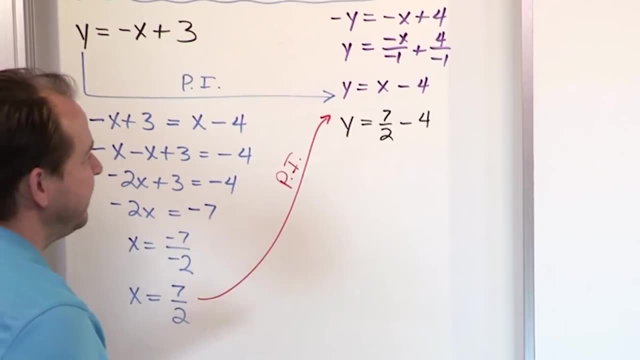 So let me go over here. and now we're saying that the corresponding value of y is equal to x, but we now know x is seven halves minus four. Now, I'm sorry, sometimes in math you just have to deal with fractions and it's not. 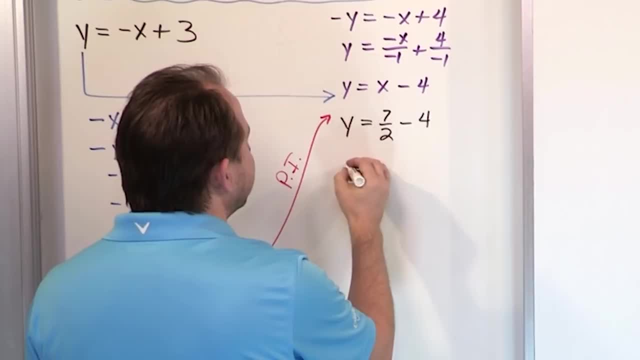 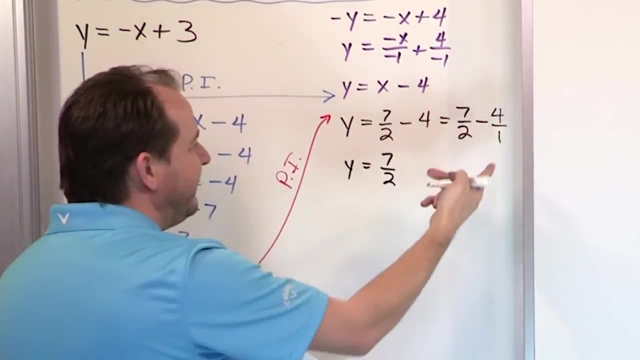 fun. I mean, I agree with you. It's not. It's not. So this means that it's seven halves and this is seven halves minus four over one. It's easier to write it like this: right Minus four over one. 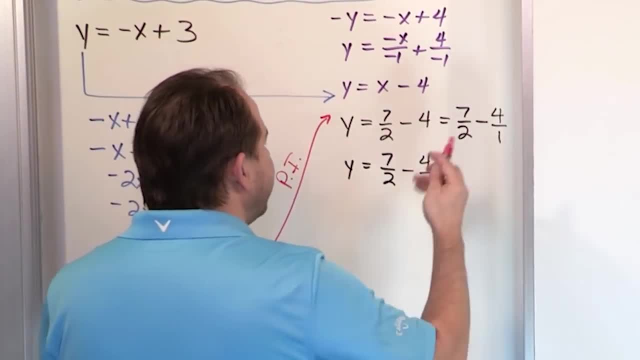 How do I get a common denominator here? I have a two and I have a one, so I can just multiply this by two on top and bottom, and that means what I'm going to get, for the y value is seven halves minus on the top. I'll 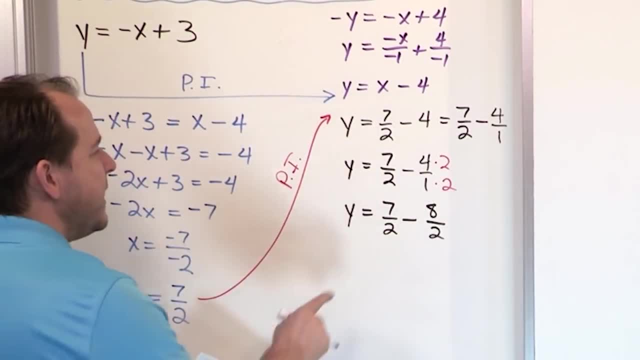 get four times two is eight. on the bottom I'll get two times one is two, And now I have seven. I have a common denominator, first of all, of two. That just goes on the bottom, and then it's seven minus eight. 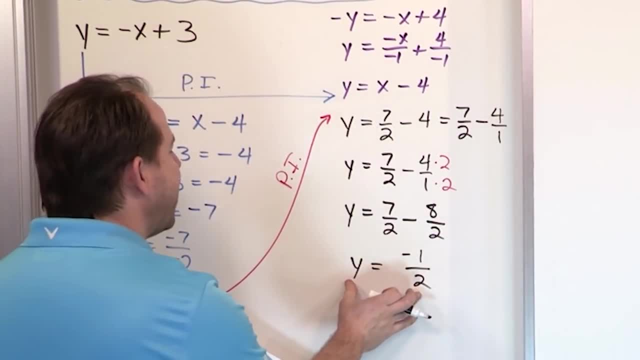 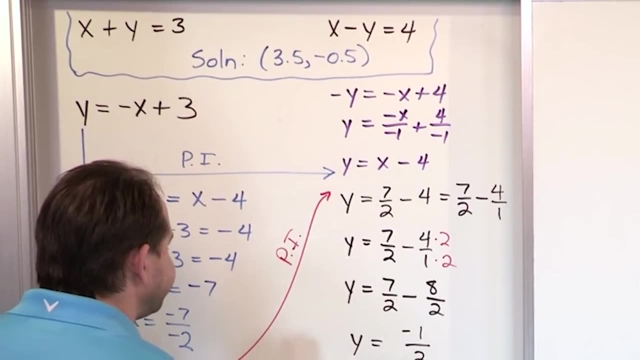 What is seven minus eight Negative one. So what do we have? The y value is negative one half, which is exactly what we got when we write our graph. So what we write down is: the solution is the x value of seven halves, or you can convert. 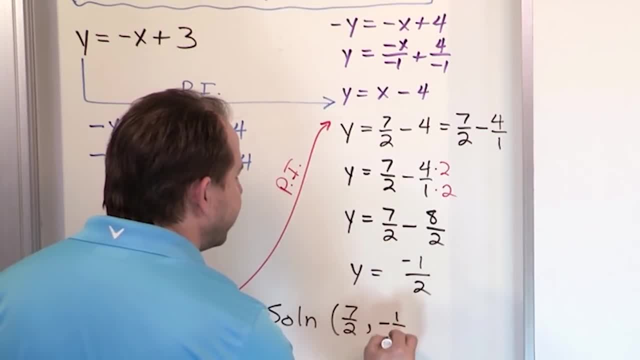 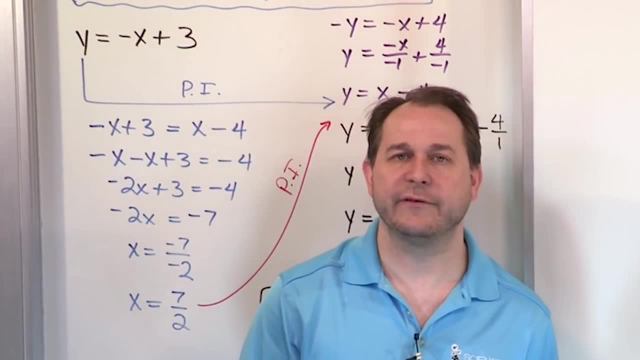 to decimal, if you like, and the y value is negative one half. This is the solution and you would write down. also, it's a consistent system, because consistent systems are ones that have solutions of intersection points. Okay, It's so incredibly important that you follow what we're doing here. 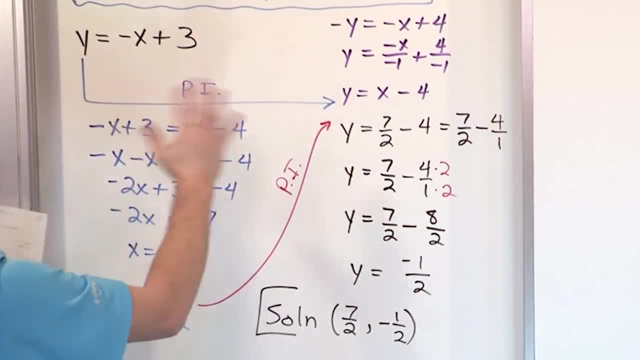 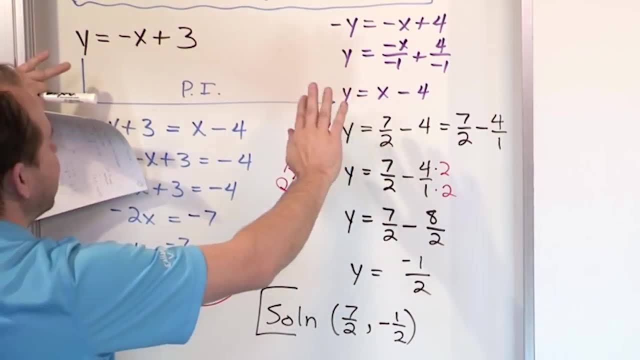 What we did is we said we have two equations. I can take one because I'm saying they have to be equal somewhere. so I'm going to take the y value of this one, I'm going to stick it into this one, But then when I do that, I eliminate y completely and I only have an equation to solve for x. 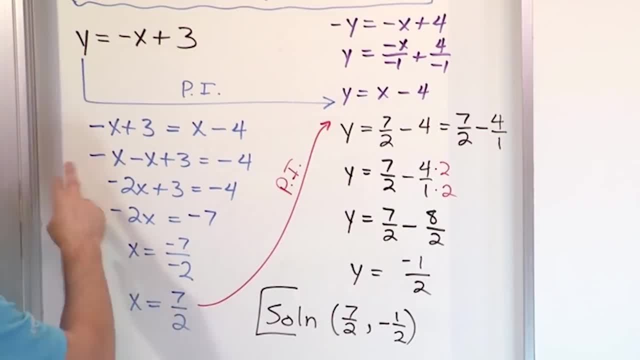 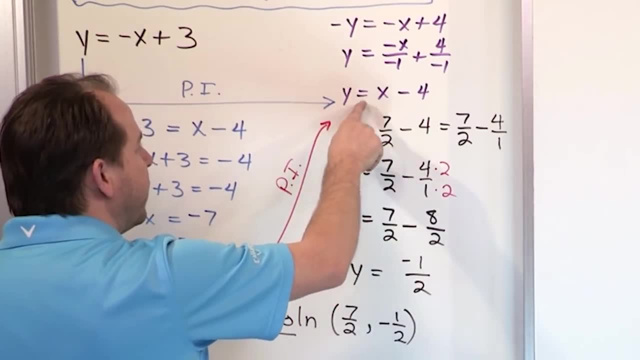 When I do the math and I simplify it down, I get the x value. that is common to both equations. Once I have that one, I substitute that in to the value for y. that will give me the value of y. I put in the value of x. 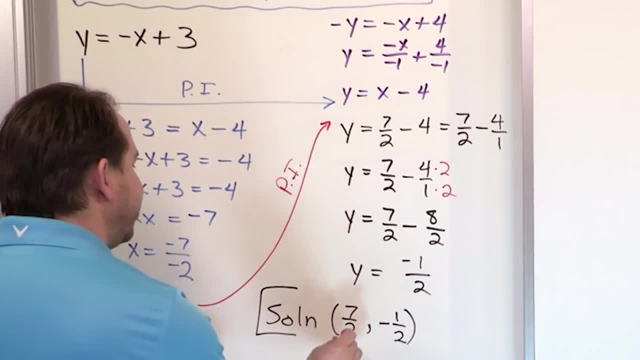 I do the math there and I get the value of y. so as a pair it is x comma y as a solution point. Now you might say: well, I can take this x value and I can stick it into here and 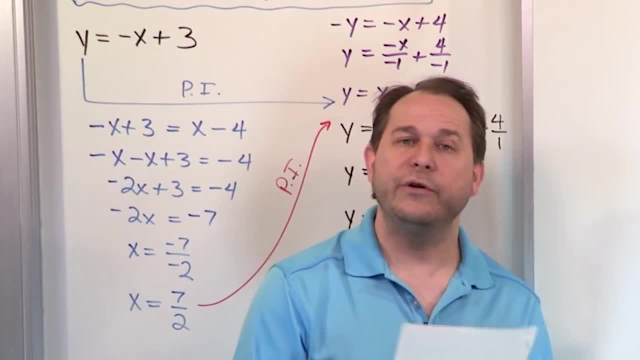 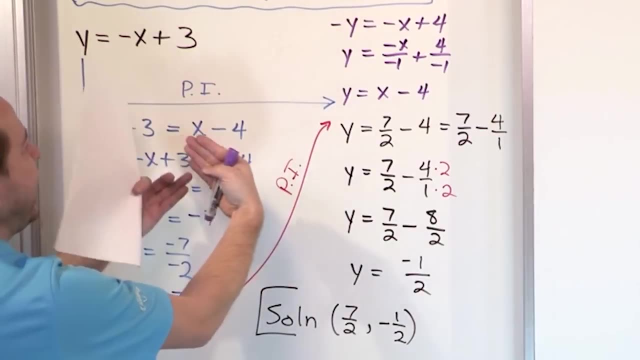 get the answer. but what I'm telling you also is that once you have the x value, you have the choice- You can stick it in here to get y, but we're saying that these are equated at that point, so you should be able to take it and also put it in here and get the same answer. 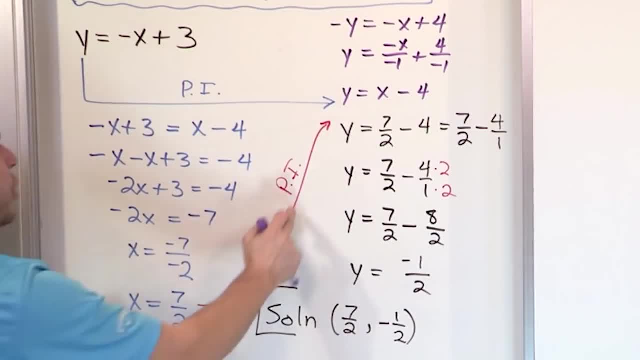 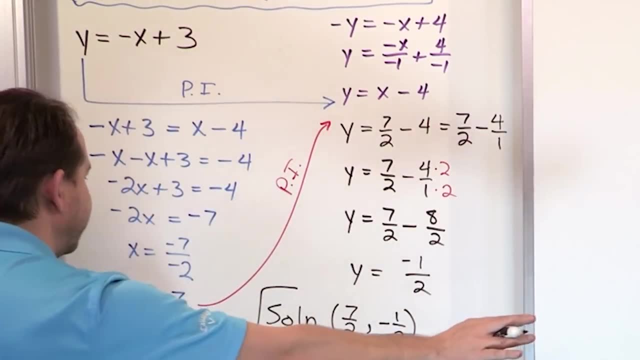 In other words, it shouldn't matter. It shouldn't matter, once I get down to half the answer, which direction I go to get the other. so let me just do it for you real quick. The solution is done, We've solved it. but now let's take this guy and put it in here. 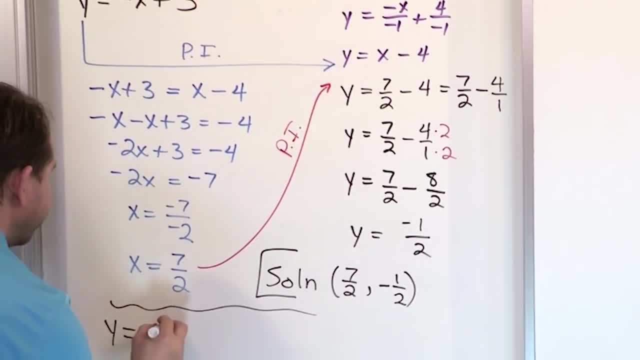 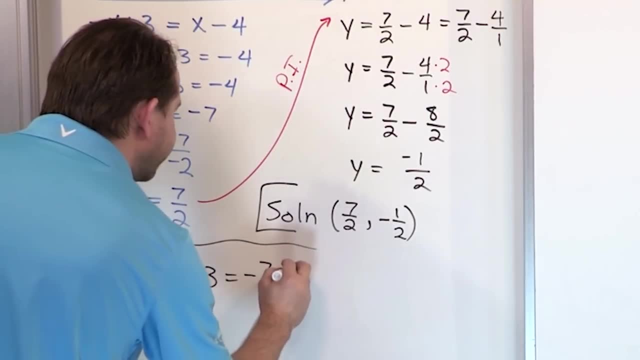 Y is equal to negative x, but x is equal to this, so it's negative 7 halves plus 3, which is negative 7 halves plus 3 over 1.. Now it's the same sort of thing to find a common denominator of 2.. 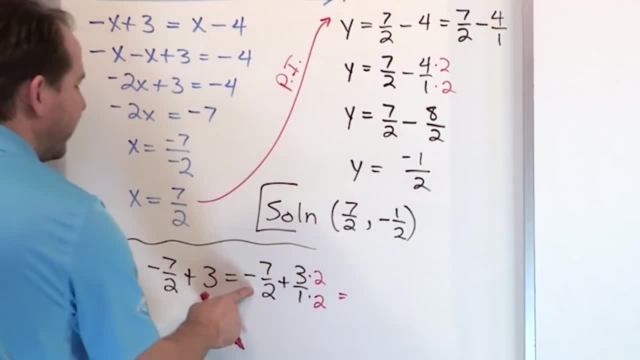 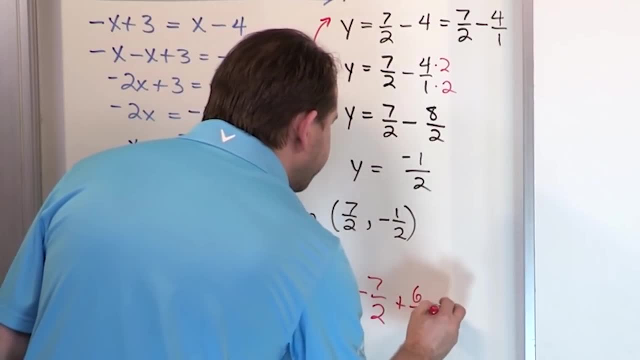 I'll just multiply this by 2.. I'll just multiply this by 2.. I'll just multiply this by 2 and this by 2, which means I'm going to get negative 7 halves, and over here I'll have 6 on the top and 2 on the bottom, which means I'll have a common 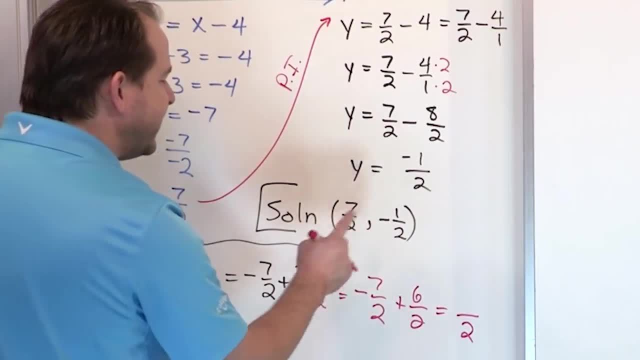 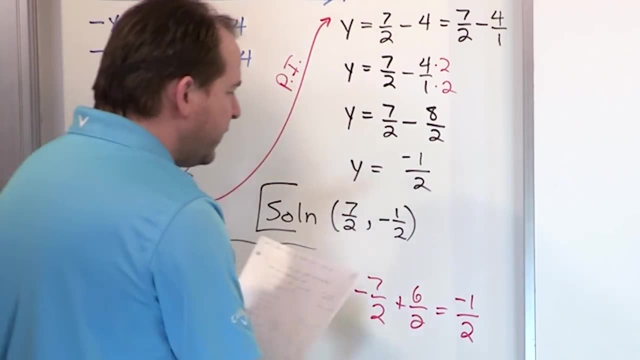 denominator of 2.. What is negative 7 plus 6? Negative 7 plus 6 is negative 1, so the value I got for y is negative 1 half. It's exactly what I got the other direction, so it's not a magic trick. 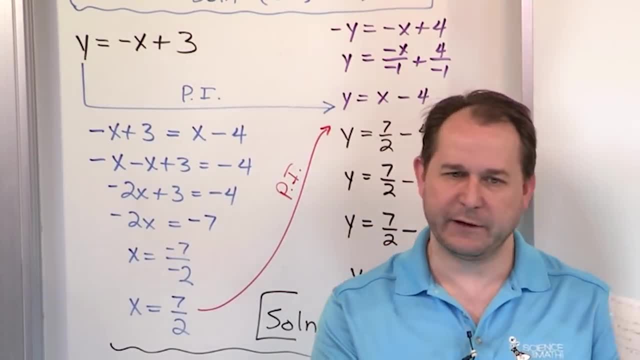 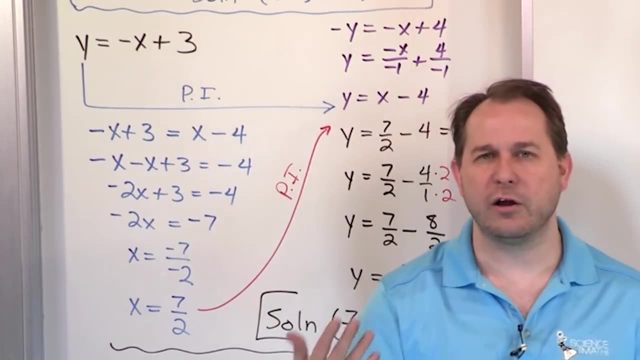 It's not like going and like somebody throwing cards and like: flip the cards, It's magic, You got the same answer. It's because we know that these lines go in different direction and we know that in all likelihood they're going to cross somewhere. 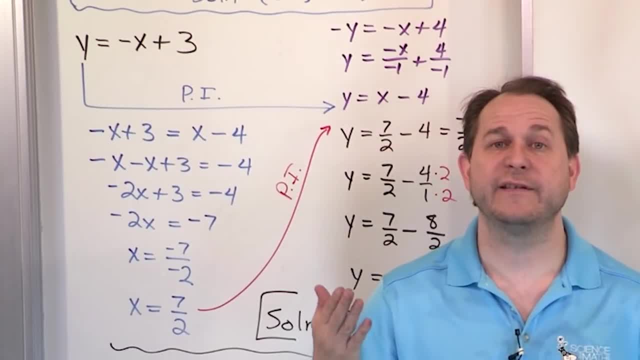 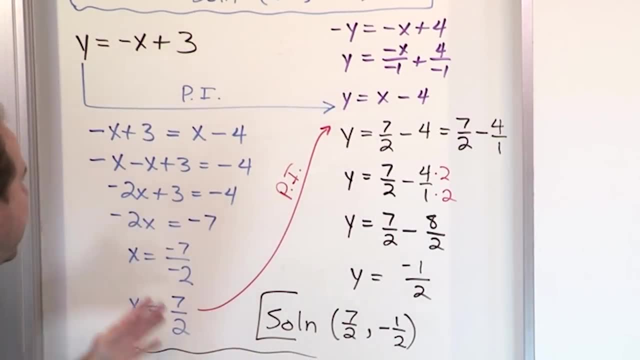 At the point that they cross, the x and the y values of both lines are the same right. That's why it doesn't matter if I put this into here or here, I'm going to get the same value because at the point of intersection the x values of 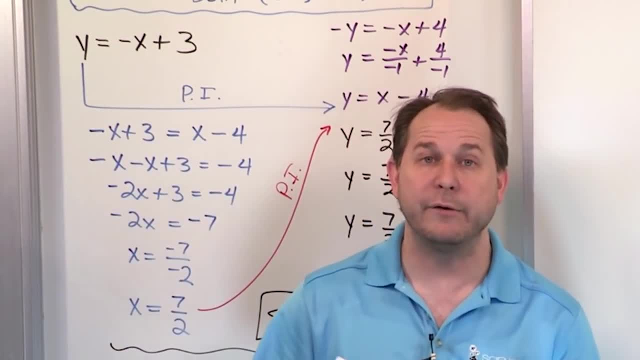 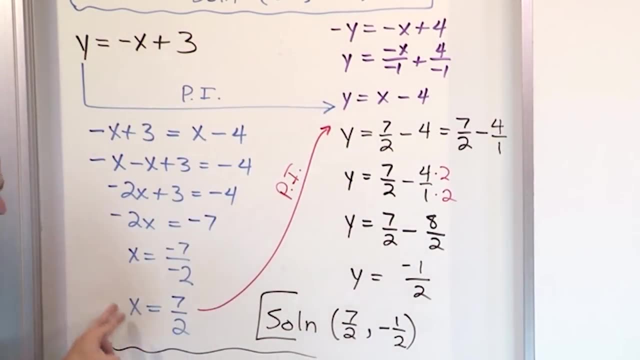 both of these lines are the same and the y values of both of the lines are also the same at the intersection point. so that's why I can take and substitute in and get the x value. I can then go back to either direction and get the corresponding y value. 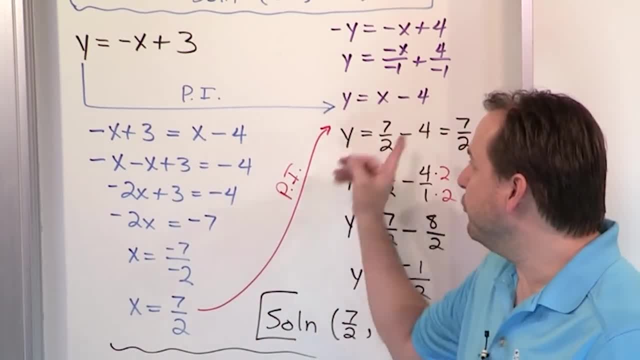 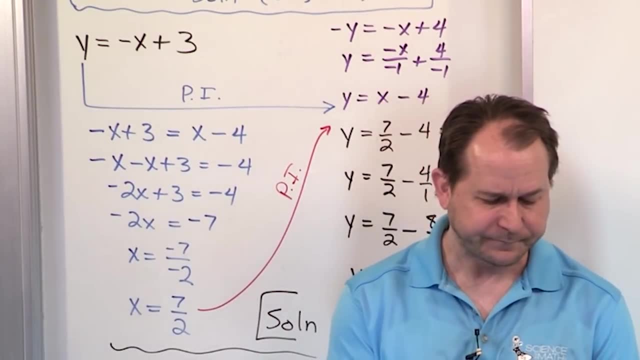 So, from here on, I'm not going to tell you, I'm not going to do both of them, I'm not going to put it in here and then put it in here and show you. Basically, you have the choice. Either way is going to give you the correct answer, all right. 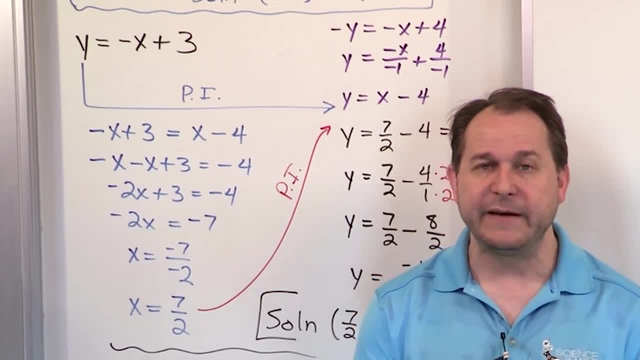 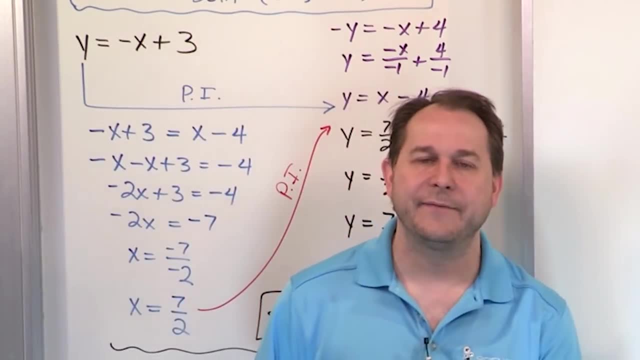 But you have some freedom in how you choose to go about doing this. Now, this is giving you an exact solution. It's giving you 7 halves and negative 1 half. This is exact. By reading a graph you're not really sure if you're right, because who knows, if I'm this. 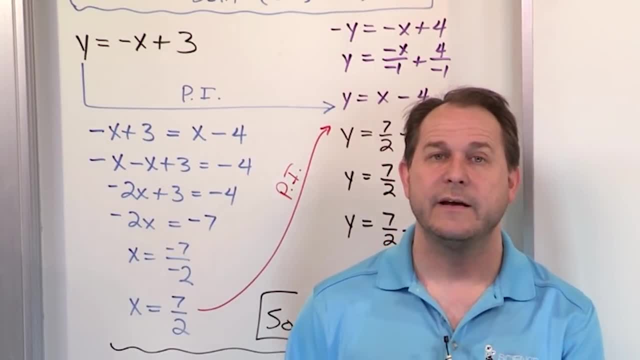 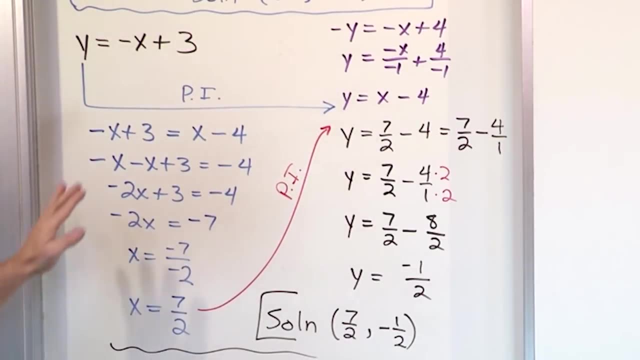 way, or am I that way? By getting an exact solution? it's exact, and you know exactly what you have. I will say one more thing: As you get down to this point, this is a well-behaved problem, meaning that you get it down, you. 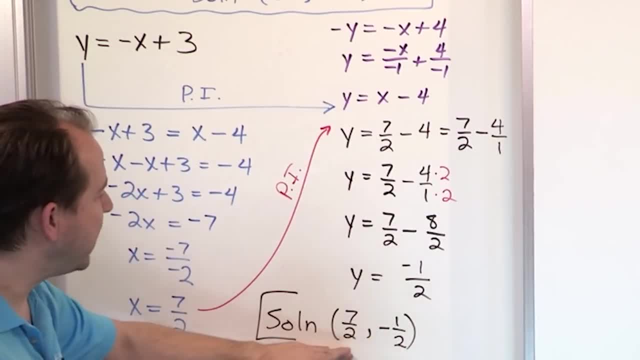 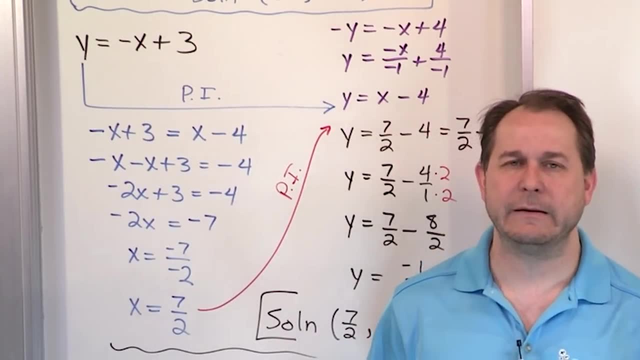 get a value of x, you put it in, you get another value of y. there's only one answer to this that you're going to get. Sometimes, when you get down and you start substituting in, you start getting weird things happen that don't look so well-behaved. 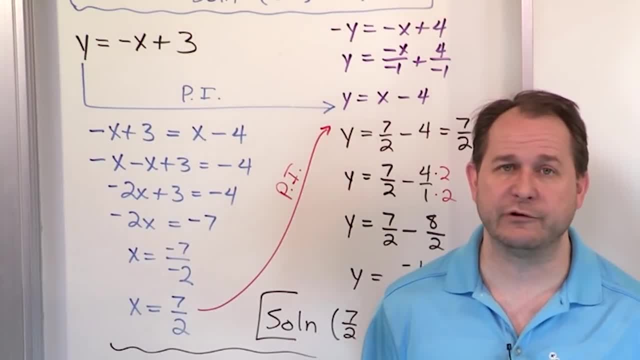 In those cases you might have an inconsistent system where there's no solution, or you might even have a dependent system where there's the lines of the basis. The lines are basically the same equation and you have an infinite number of solutions because it's the same line. 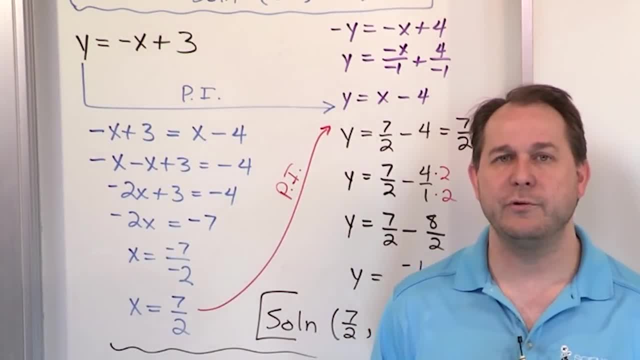 Both of the equations are the same thing. As we get to those problems, I will show you how to identify that. I'm not sure if we have any in this lesson or not. let me just check real quick. We have one coming up later where there's no solution at all. 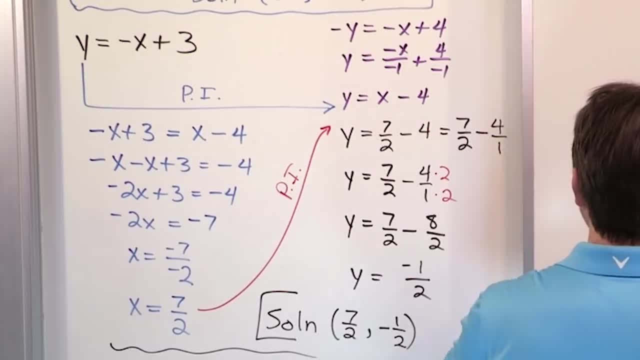 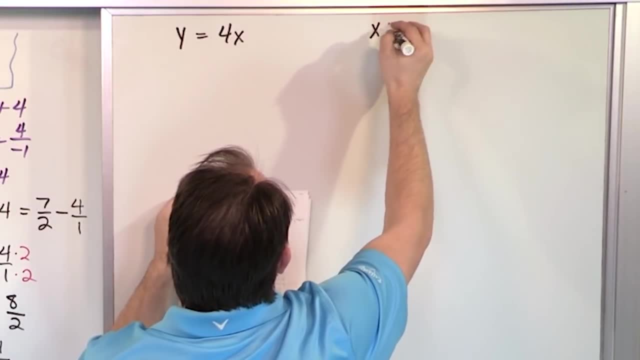 For now, let's go on and move along and try to solve another one to get some practice. Let's say we have the system of equations: y is equal to 4x and we have the other equation, x plus y. Y is equal to 10.. 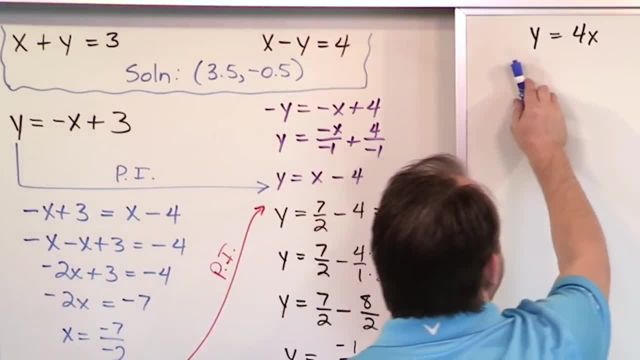 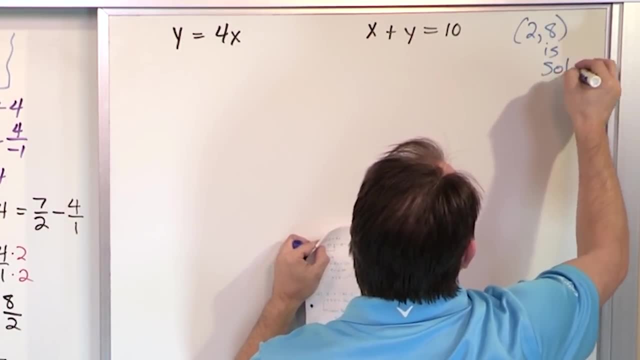 Now, actually we've already solved this one also. This is one that we solved by graphing. We know already that 2 comma 8 is the solution, but I'm not worried about giving you that, because if you just circle this on your test, nobody's going to give you any credit. 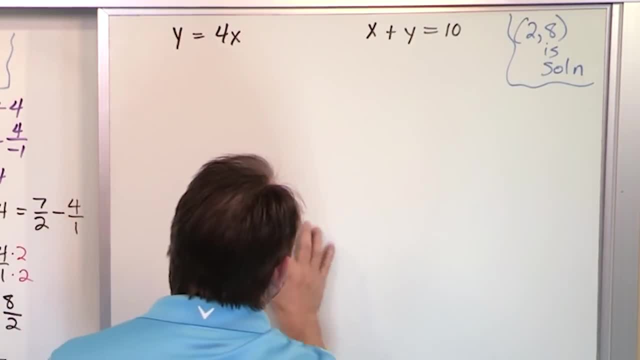 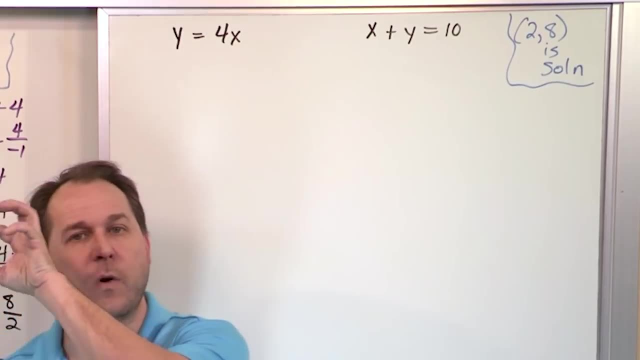 Nobody cares if you can write down an answer. What I care about is if you can do it and show me how you did it. What's the strategy here? The strategy for solving systems of equations by substitution is just to take one equation and substitute it into the other one, then solve for what you can get an answer and 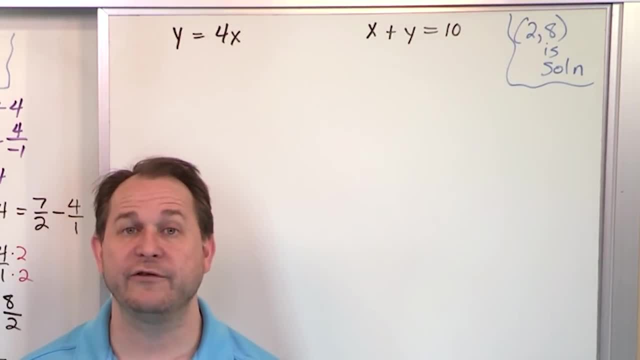 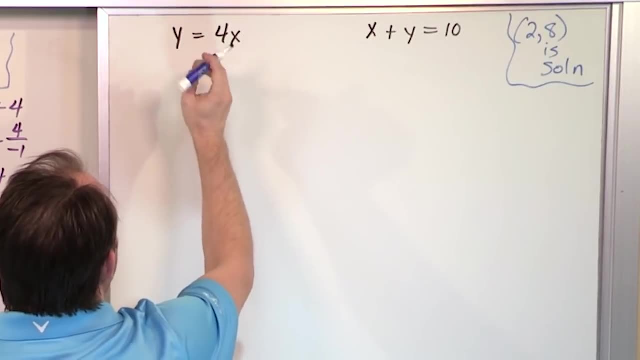 take that answer and, backward, substitute it into one of the first equations to get the other half of the answer. That's pretty much the roadmap for every one of these. So, since this equation is already solved for y, what I'm going to do is I'm going to plug. 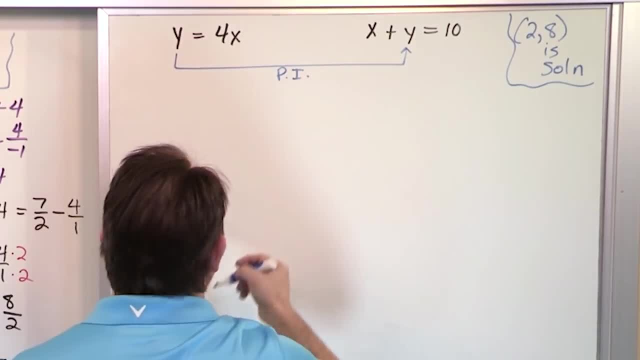 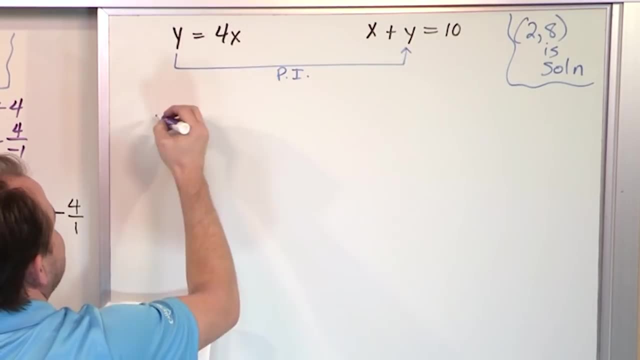 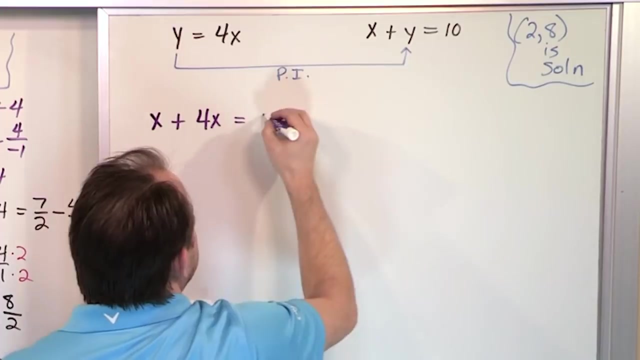 it in for this value of y. I'm going to plug it straight in, So what I'm going to have is over here. if I were to work and pull that down here, it'd x plus y, but now I'm saying y is actually equal to this, for x is equal to 10.. You see how all I 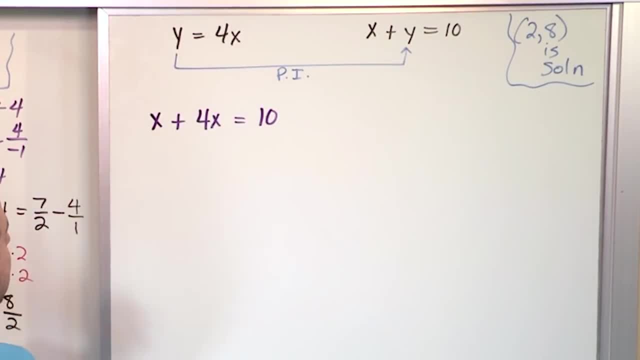 did is: I took this value and I just stuck it in where it should go. Now, what do I have is 5x equals 10.. Now, what do I have is 10 over 5, because I divide by 5, x is equal to what? 2.. 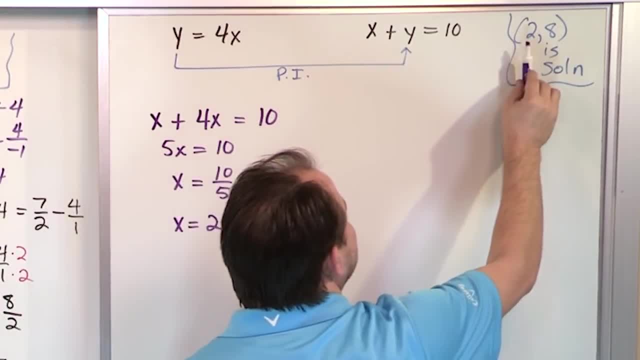 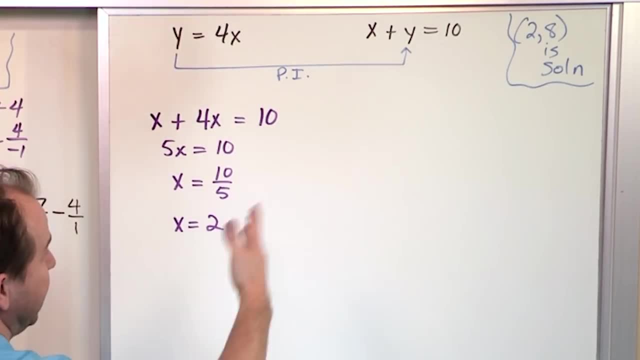 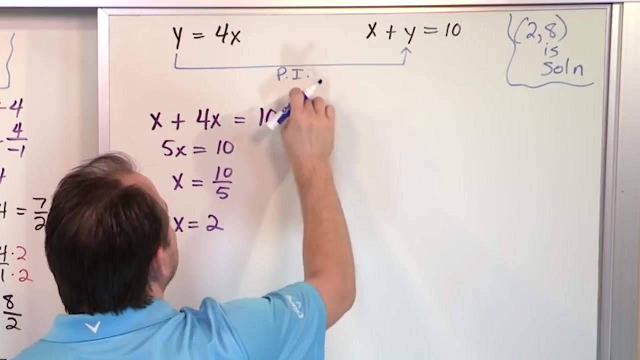 So I'm saying the x value of the intersection point is 2, which is exactly what we found by graphing The x. the x, the value of the guy is equal to 2.. Now, or the intersection point is equal to 2.. Now we take this half of the solution. we have a choice. Let's stick it into the easier. 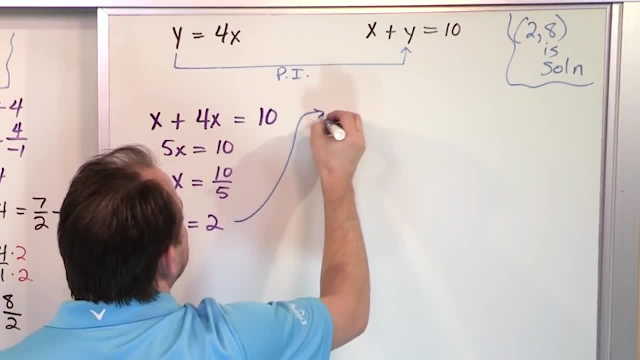 one. This is the much easier equation to deal with. So I'm going to go over here and I'm going to say: y is 4x, because that's what. that's what I'm given. So y is 4 times what is x. We now 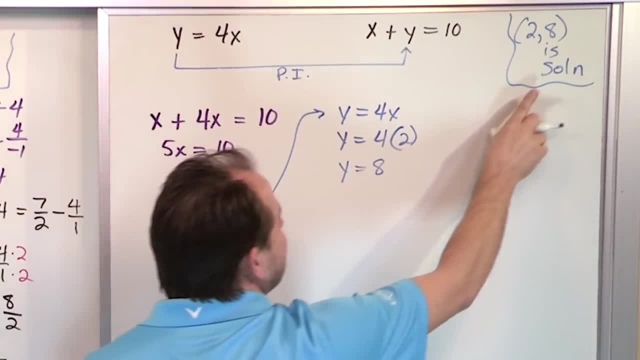 know x to be 2,, so y is 8.. And this is exactly what we got here. So then we say: what we know is that 2x is equal to x. So we now know x to be 2,, so y is 8.. And this is exactly what we got here. 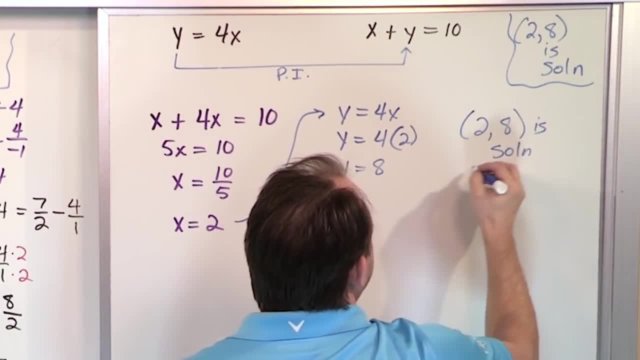 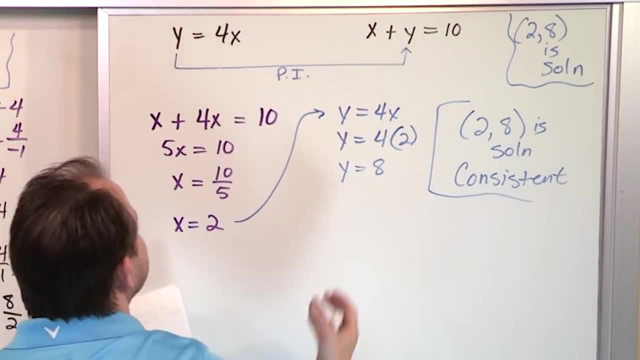 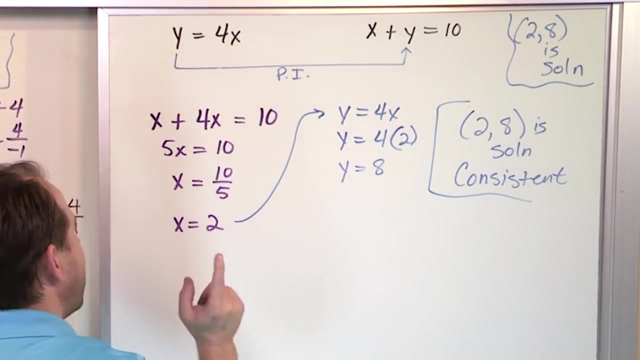 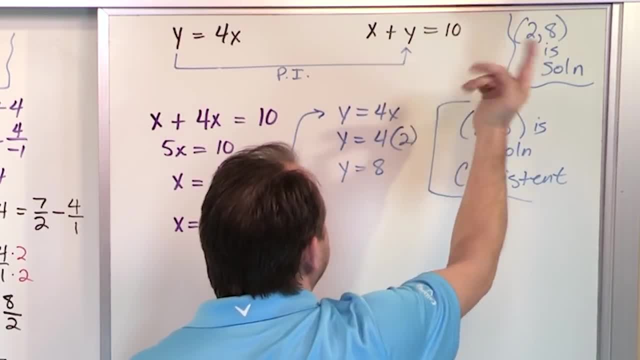 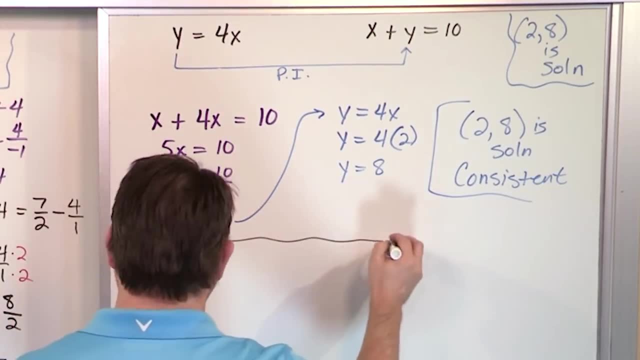 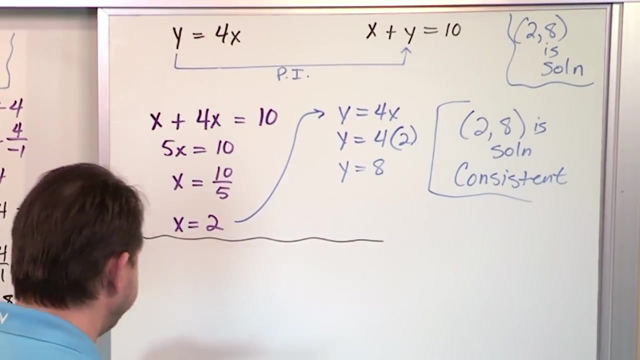 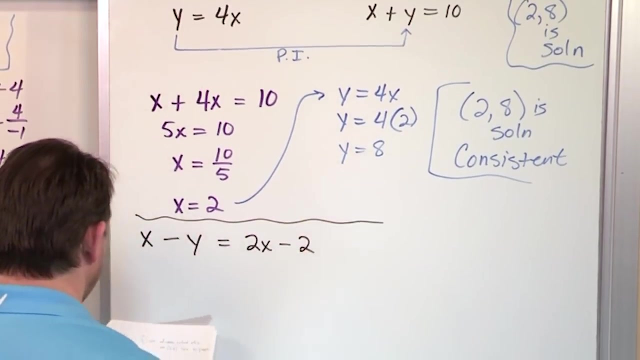 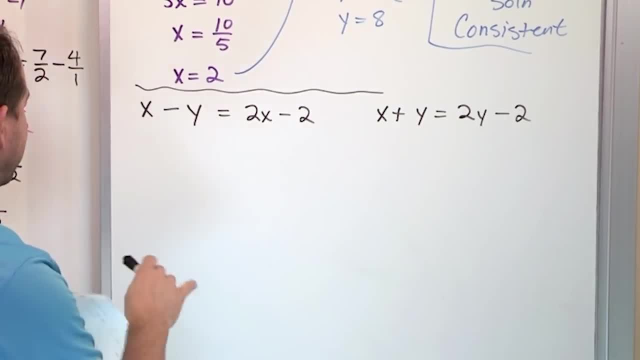 minus 2.. So they look similar. but don't be fooled. You have x minus y on the left. you have x plus y over here, You have 2x minus 2 and 2y minus 2 there. So you don't yet know. is this consistent? is it inconsistent? does it have a solution? 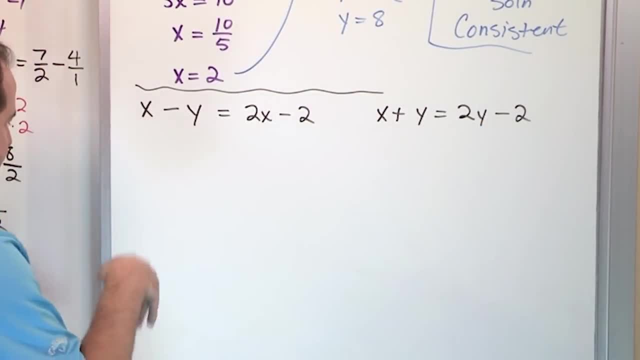 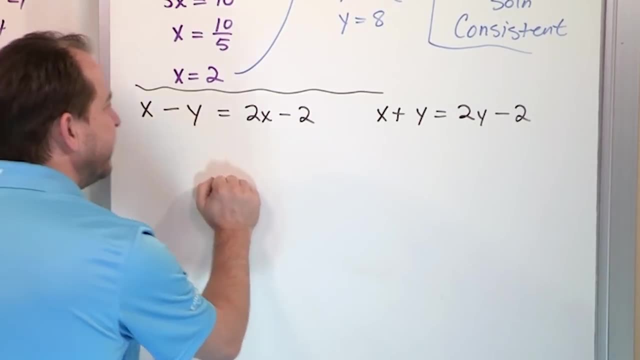 Nobody can look at this and tell you: oh yeah, yeah, I know what that is. Nobody can. If they tell you they know that, then they're just fooling themselves. What we have to do is find something in this equation to substitute into here, or I can. 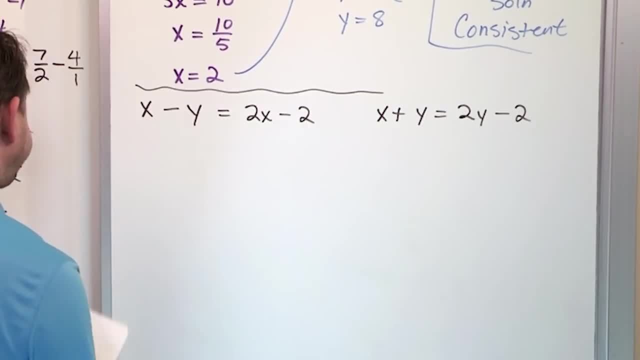 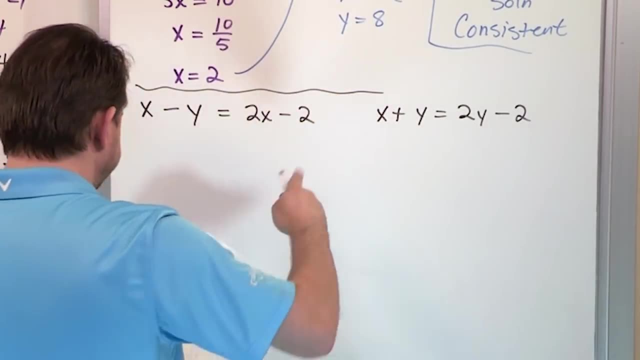 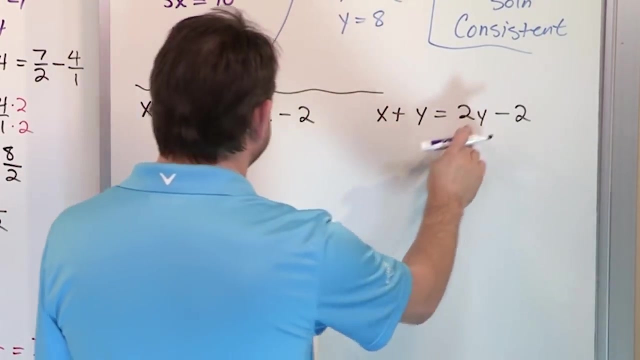 go backwards. I can find something here and substitute in over here. Let's first. I'm just going to pick something at random. Let's just work with this equation and let's solve it for y. Let's just solve it for y, so we'll substitute it back in over here. 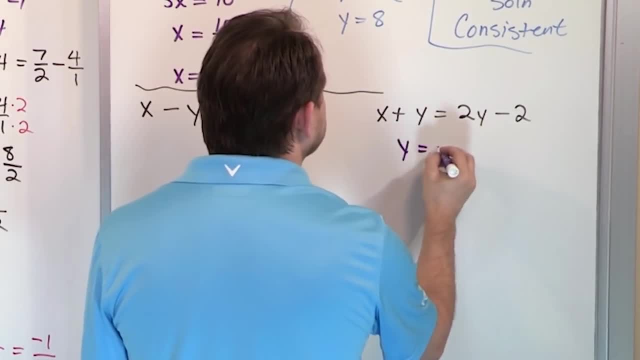 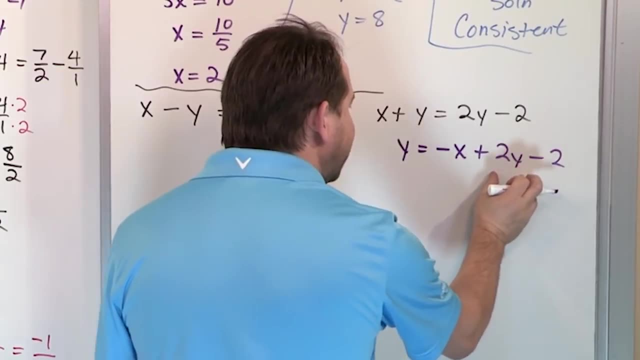 So what am I going to have? Let's move x over here first of all. so it'd be: y is equal to negative x plus 2y minus 2.. I just take the x and move it over by subtraction, And now I have a y over here. 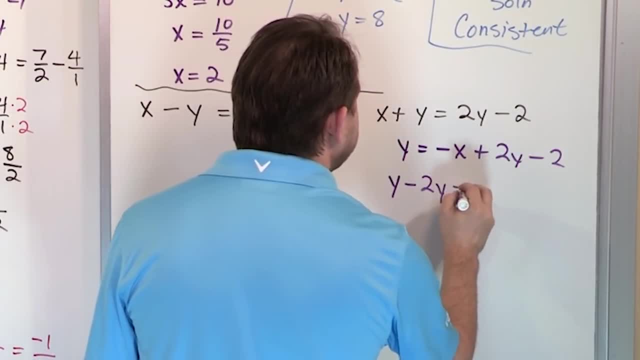 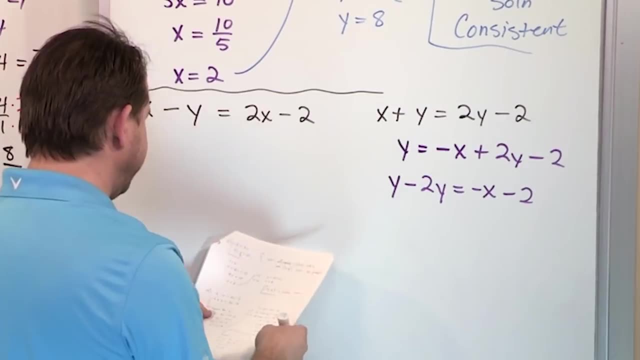 I need to move him over. so it'd be: y minus 2y is negative, x minus 2.. I just subtract 2y, subtract 2y. Now this becomes 1 minus 2.. What is 1 minus 2?? 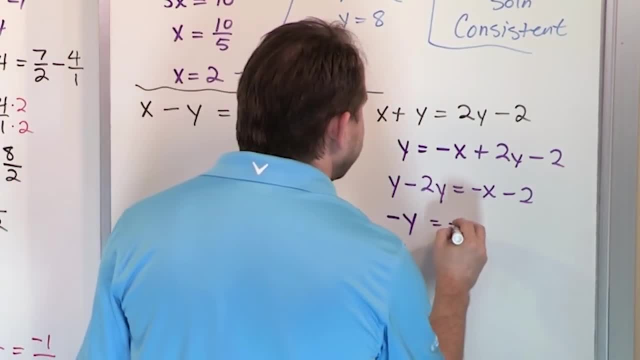 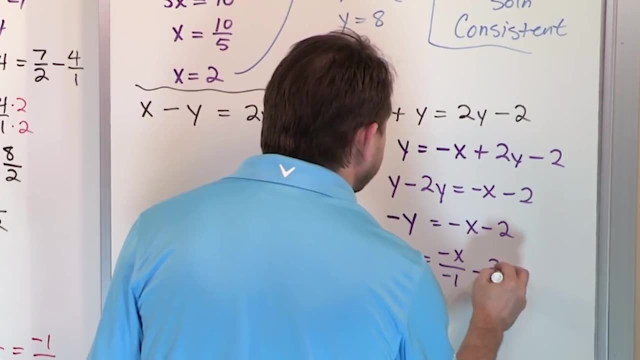 It's negative 1. So it's negative 1y equals negative x minus 2.. Now to get y by itself, I have to divide by negative 1.. So negative x over negative 1 minus 2 over negative 1.. 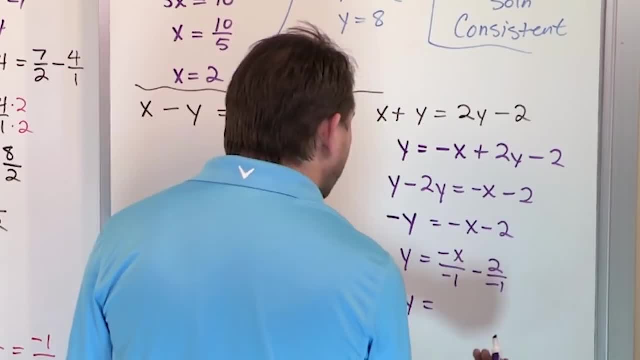 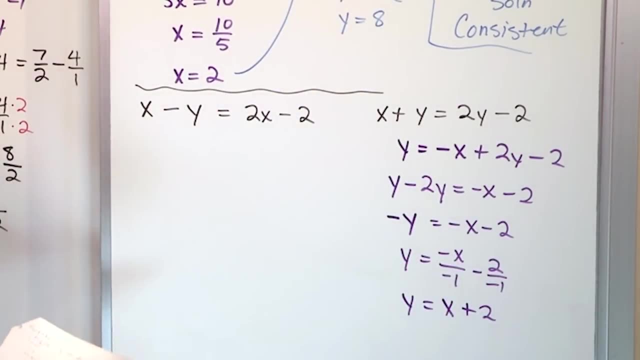 Just divide each term by negative 1.. And so what I'm going to get for the y value is going to be positive x. This would be positive plus 2, right? So I have x plus 2 here. Why did I do all that business of solving for y? 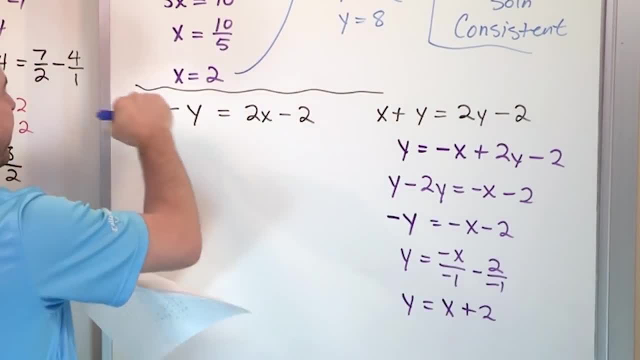 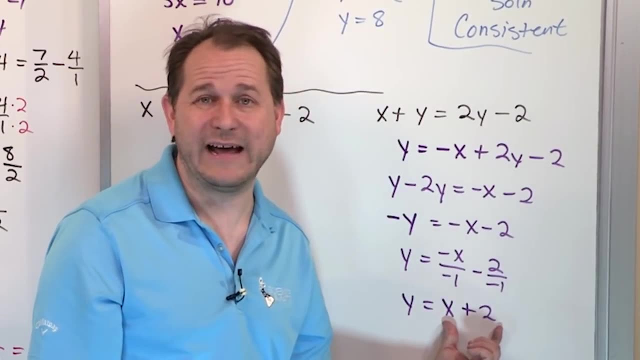 Because I have to take something from one equation and solve it, I mean plug it into the other. So that means you have to solve for something initially that you know what it's equal to. I don't really know the answer, but I know it's equal to x plus 2.. 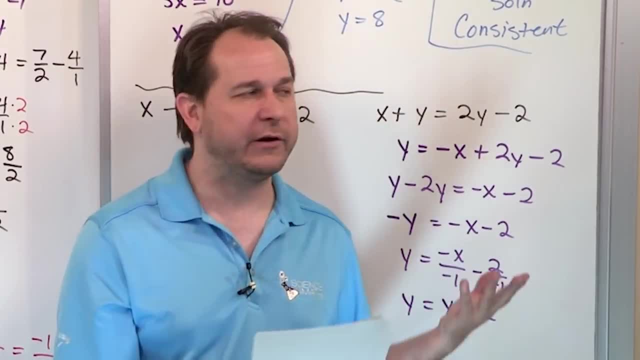 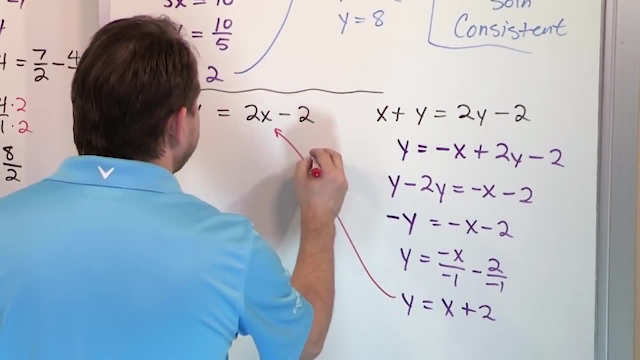 And then I'm going to stick it into all the locations in the other equation where y is prevalent or where y is. So what I'm going to do is I'm going to go up here, I'm going to go and say: plug in. 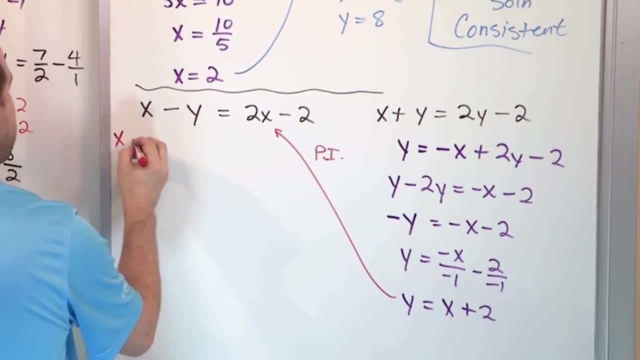 That's what the pi means, And so what I'm going to have is x minus y, but I'm going to have to wrap it in parentheses, because now I know that y is x plus 2.. It's important for you to wrap things in parentheses because if you don't, you will make sign errors. 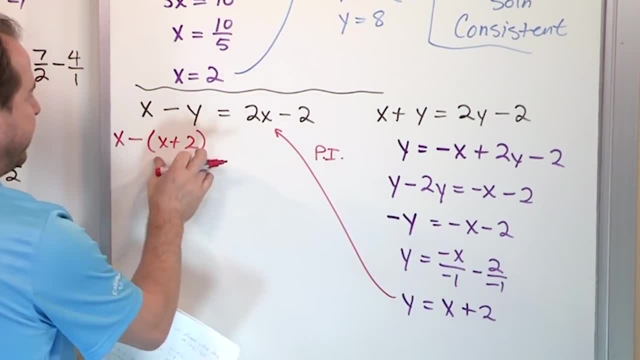 You're subtracting the value of y, which is a big expression, So put it in parentheses- equals 2x minus 2.. So on the left-hand side you're going to have x, Here you have a negative 1.. 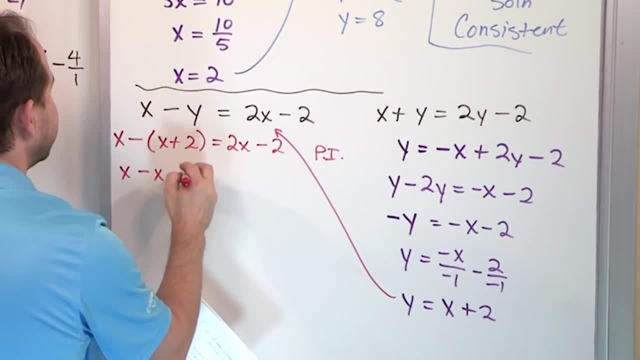 Negative 1 times x. Negative 1 times x is negative. x Negative 1 times 2 is negative 2.. 2x minus 2.. Now I have to collect all the x's. But the interesting thing about it is on the left-hand side I have x minus x. 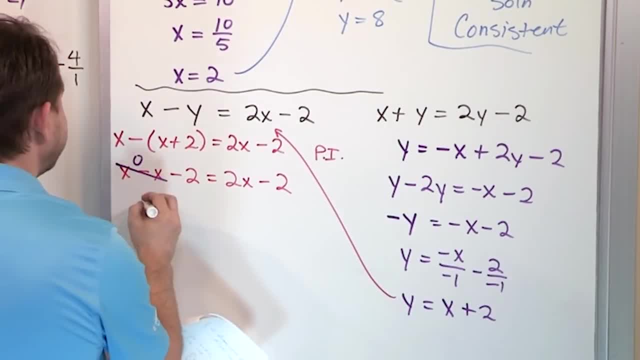 That's just 0. It goes to 0 right here. So on the left all I have is negative 2 is 2x minus 2.. So just to make it a little easier, let me leave the x on the right and let me pull the. 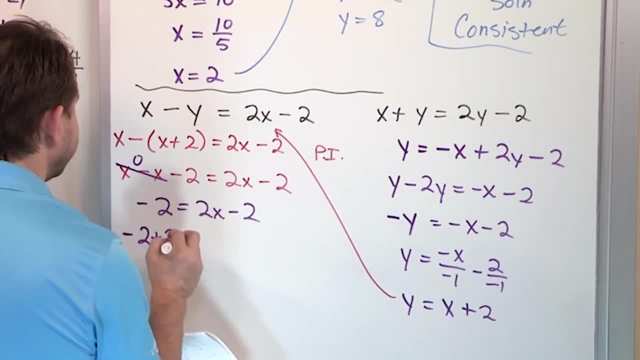 2 over by adding, So it'll be as negative. 2 plus 2 on this side equals 2x. All I did was add 2. And add 2.. But on the left that means I have 0 is 2x. 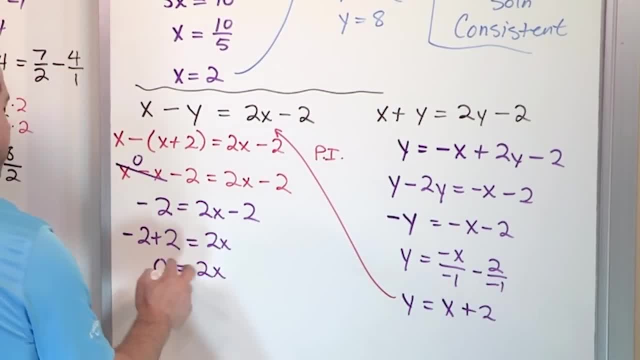 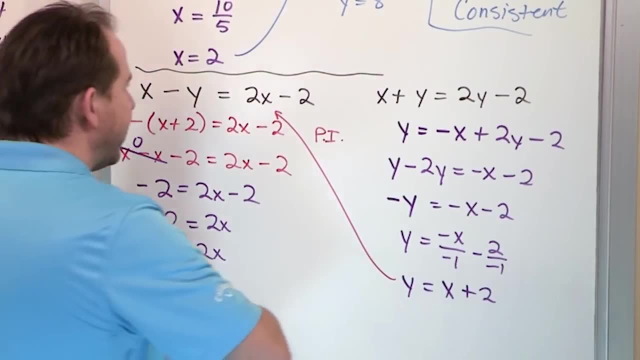 Now, if I want to get x by himself, it'll be 0 divided by 2.. So what I've said is that x is equal to 0.. All I've done is I've taken something from the right-hand equation, I've grabbed it. 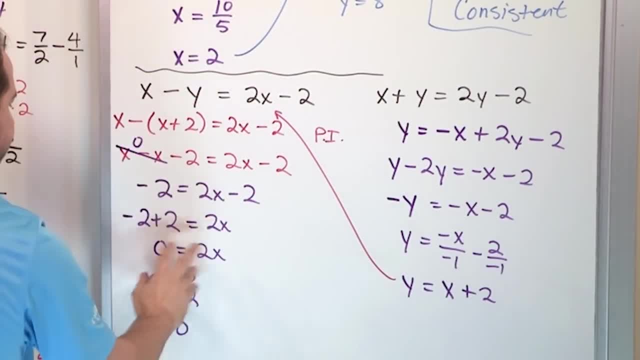 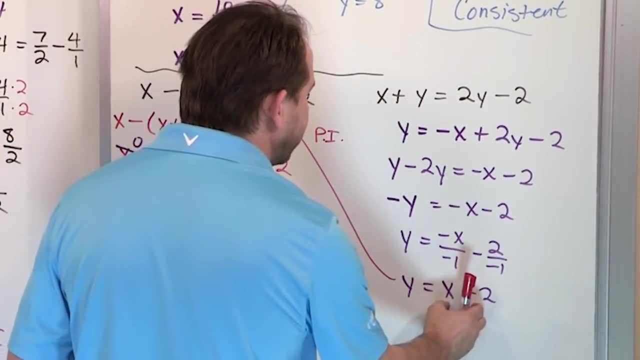 I stick it in the value where it goes, and I've simplified and solved everything down so that now that I know what x is equal to, that's half of the answer. Now I have a choice: I can take this value and I can stick it into this equation. 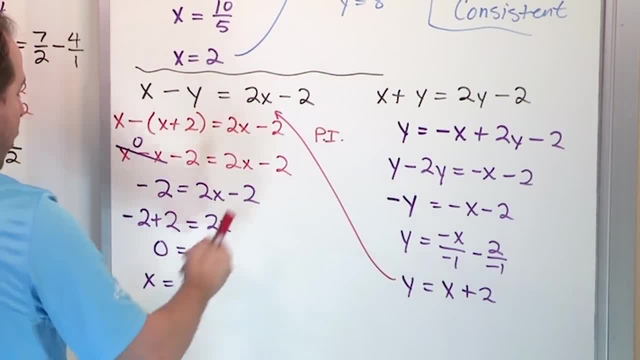 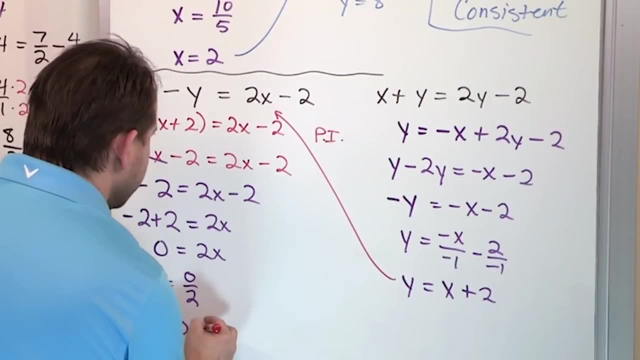 Or I can take this value and stick it into this equation, one of the original two, Or I could take it and I can stick it into the original one here, but I've already manipulated this one, so this is a much, much simpler place to go. 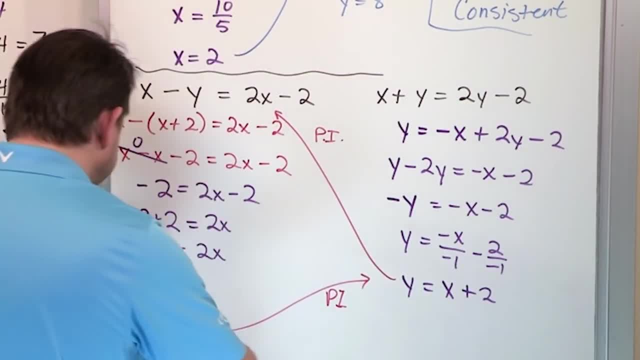 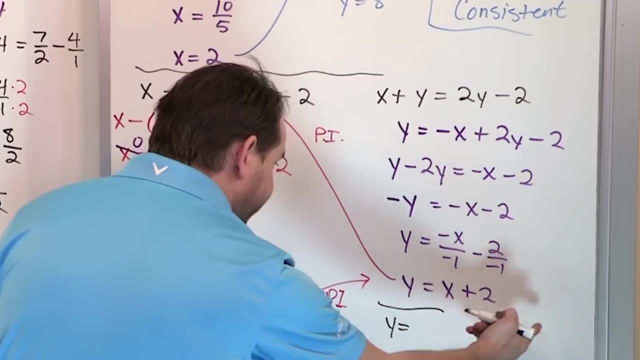 So I'm going to go this way and I'm going to plug it in here. It doesn't matter which way you go, you're going to get the same answer. So what happens is you get that y is equal to x plus 2, but now we know that x is 0. 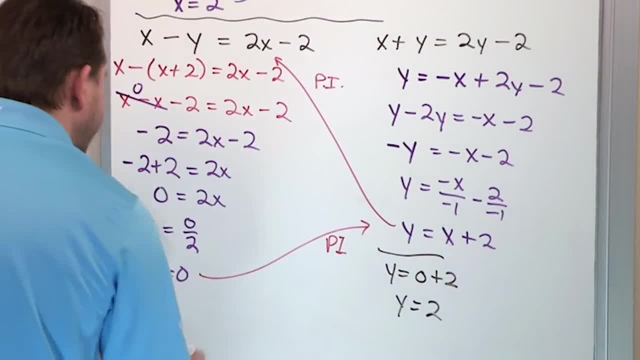 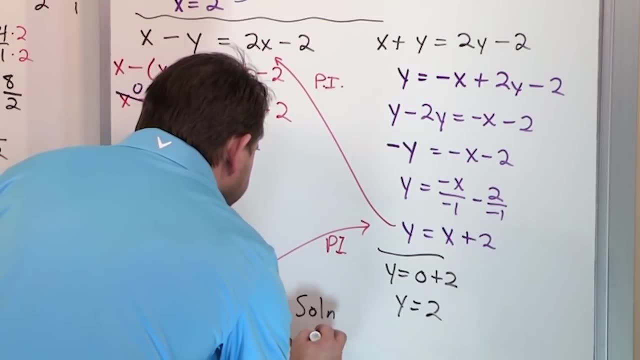 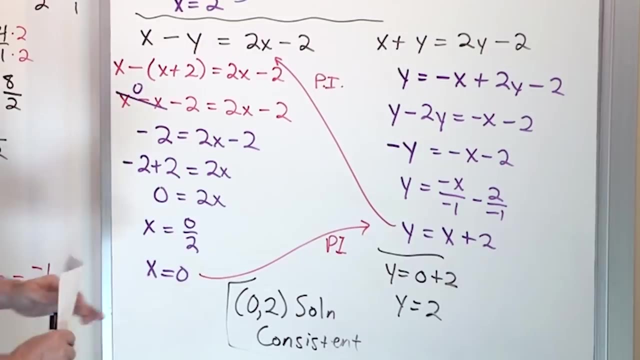 Plus 2, so y is equal to 2.. So what you write down in your paper is 0.. 2 is the solution, and you say it's consistent, Consistent, all right. So if you were to take this value of 0 and stick it in here, what would you get? 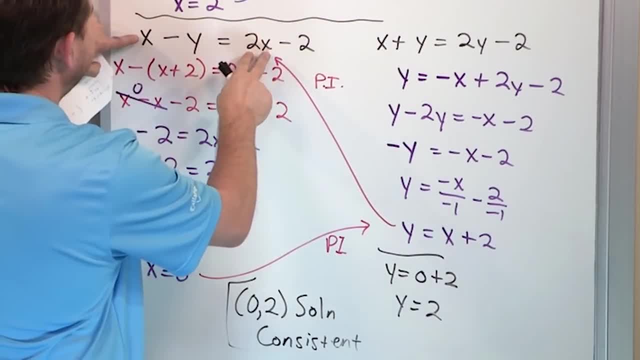 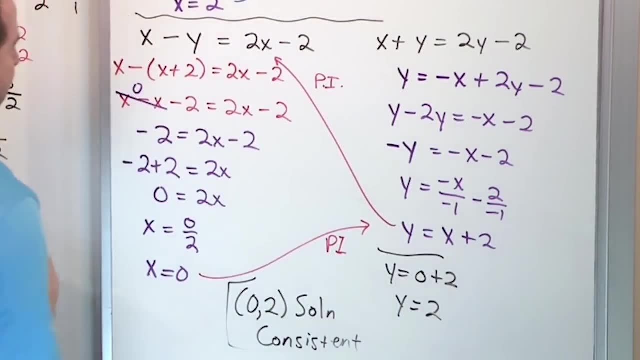 Well, it would be 0 for here, 0 for here. These two terms would drop away completely. You would have negative. y is equal to negative 2.. You would divide so you'd say y is equal to 2, exactly what we got before. 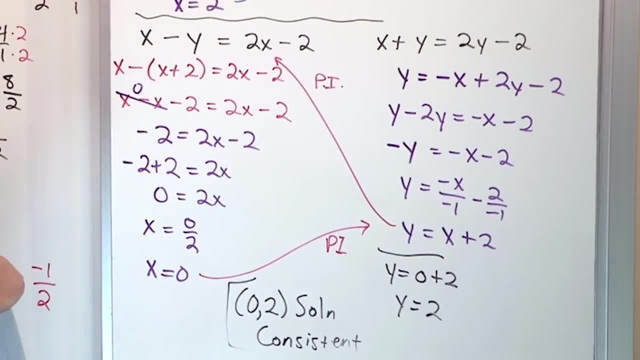 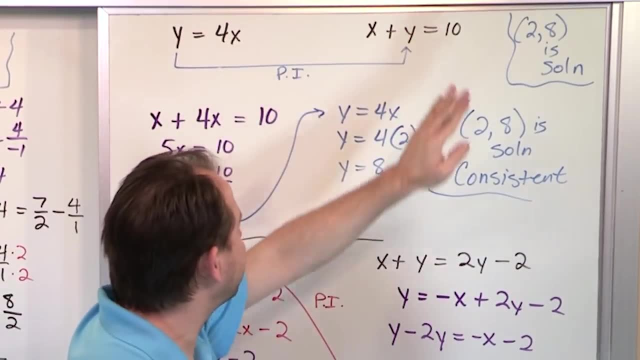 All right, So this is a consistent system. All right, so so far. if you were to graph this and graph this, you would find they would intersect exactly at this point. If you were to graph this and you were to graph this, you would find that they intersect. 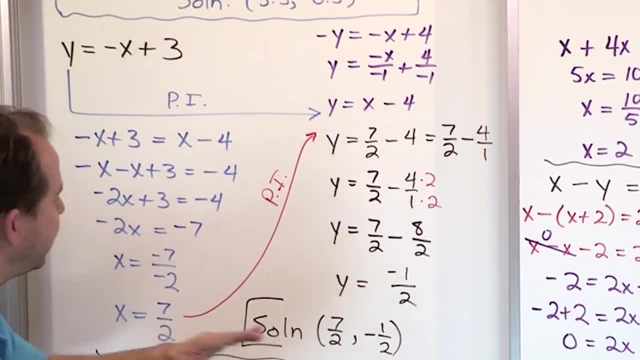 at exactly this point. If you were to graph this and graph this, you would find that they intersect at exactly this point, And in fact we've actually solved a lot of those already, so we've already done the graphing for a lot of them. 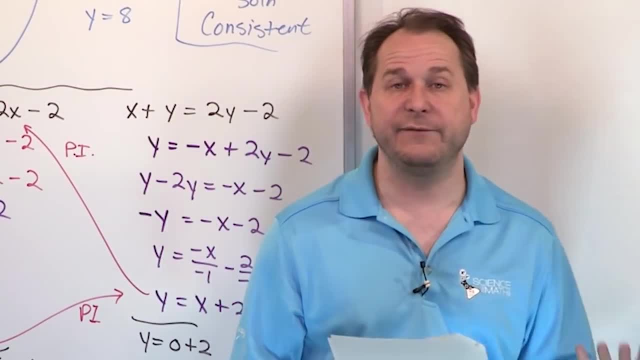 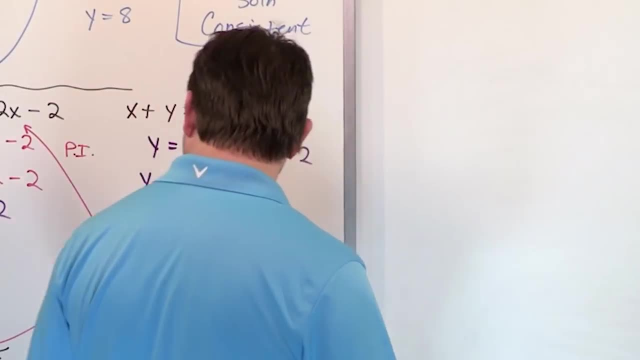 Now what I'd like to do is show you what a set of equations looks like when it's not well behaved, it's not consistent. It's kind of like how you identify what to do and so on, as we go on down the road. 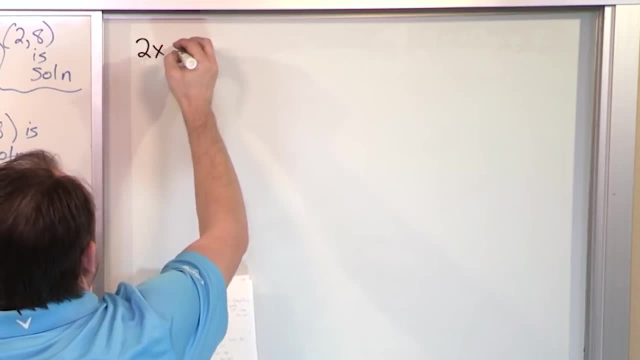 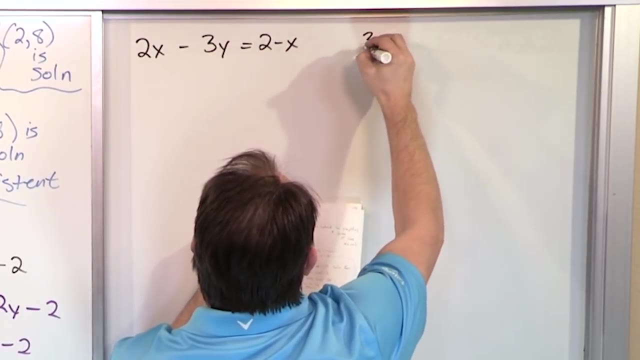 So the system of equations we're going to have for our last problem is: 2x minus 3 times y is equal to 2 minus x, And the other equation is going to be: 3x minus 2y is negative: 2 plus y. 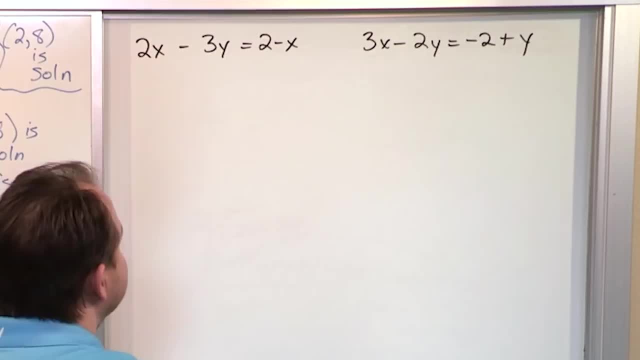 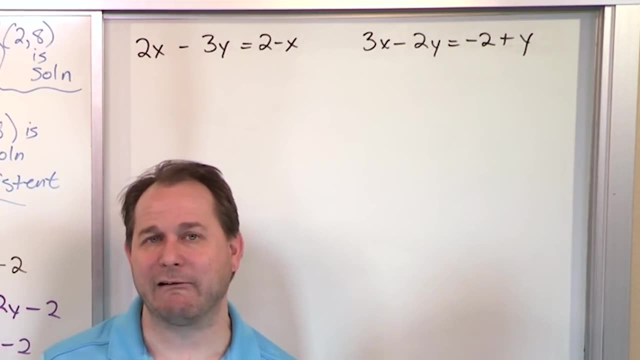 All right, Now we've already actually solved this set before as well, So if you go back to the graphing method, you'll find that we've already graphed them. These lines turn out to be parallel, All right, So let's go and work through it through substitution and just see what it looks like when two lines 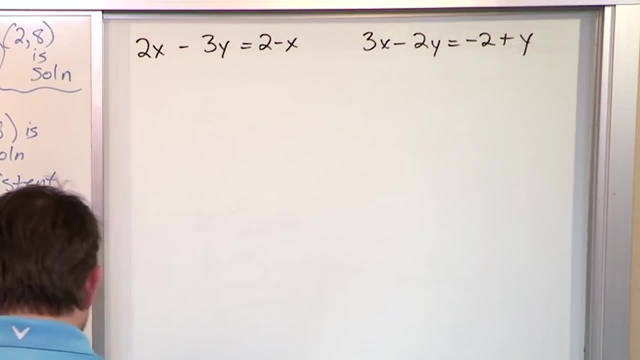 don't have a solution because they're parallel, right? So, first of all, this equation has a bunch of stuff all over the place x's and y's. and this equation has a bunch of stuff all over the place x's and y's. 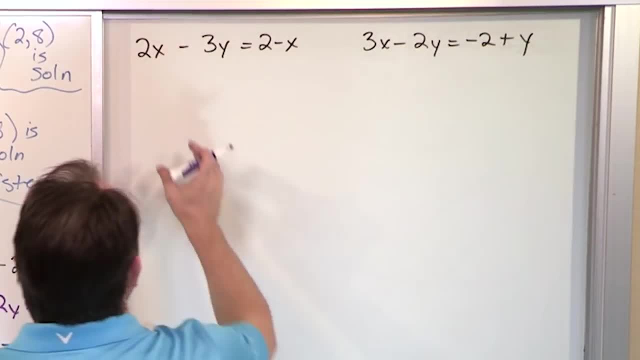 So the first thing we're going to want to do is clean them up. So what I'm going to do here- what I mean by clean them up- is try to get the x's and y's off to one side there. So let's put it in standard form. 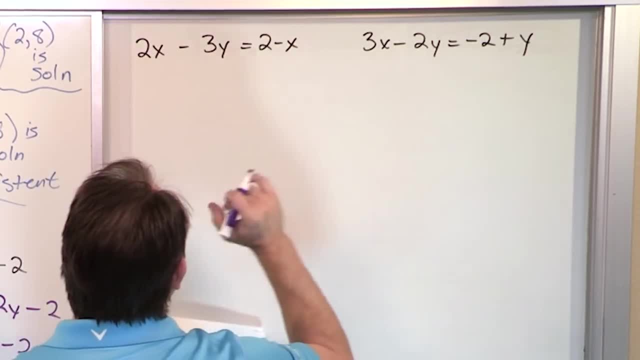 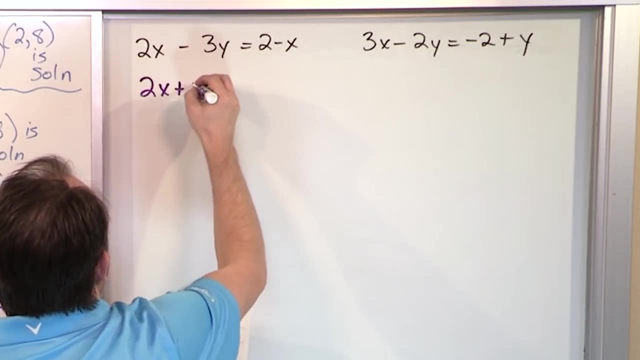 Let's get the x's and y's on one side. We can do it many, many different ways, but let's do it this way. Let's move the x over here. So what we're going to have is 2x. we're going to add x, so it'll be plus x minus 3y equals. 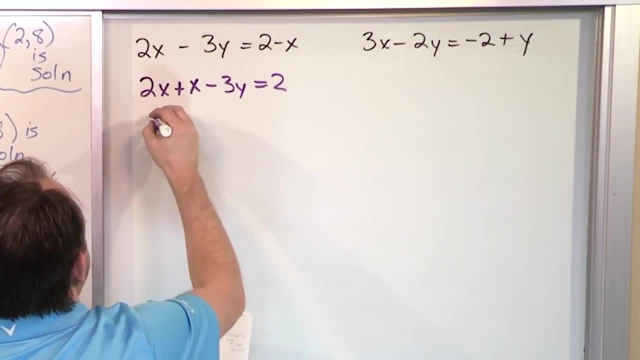 2. I just added x and I added x, so this becomes 3x minus 3y equals 2.. I could put it in an mx plus b form. That's totally fine, but let's just do it this way, just to do something a little bit. 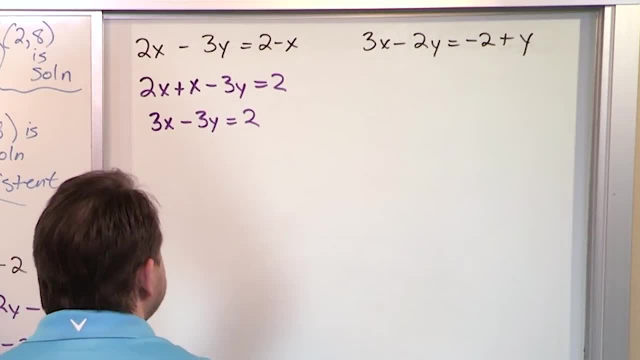 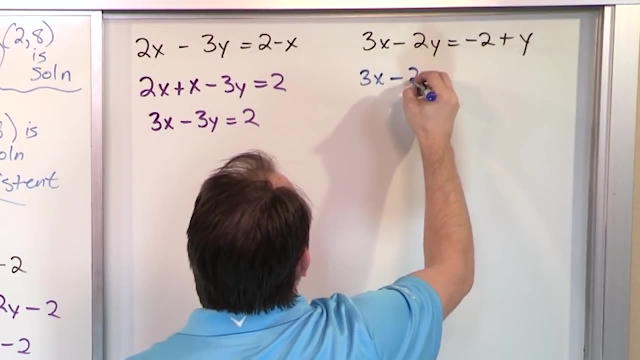 different. All right, Now for this guy over here. Let's put it in standard form also: Let's move the y over here, So we'll have 3x minus 2y. We're going to subtract. y means we're going to subtract another y is negative 2.. 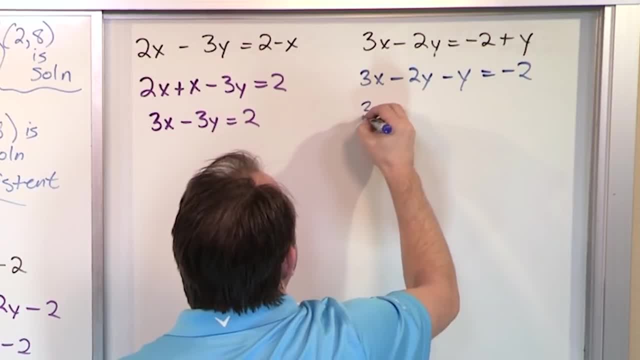 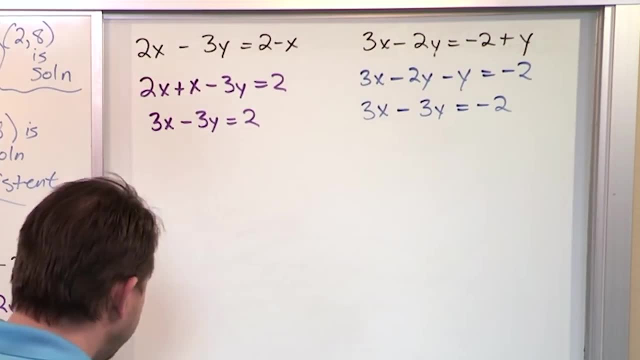 We subtracted y, we subtracted y Over here we're going to have 3x minus what's minus 2 minus 1 is minus 3y. negative 2 is the answer. Okay, So now we're down to the point where we need to solve for something. 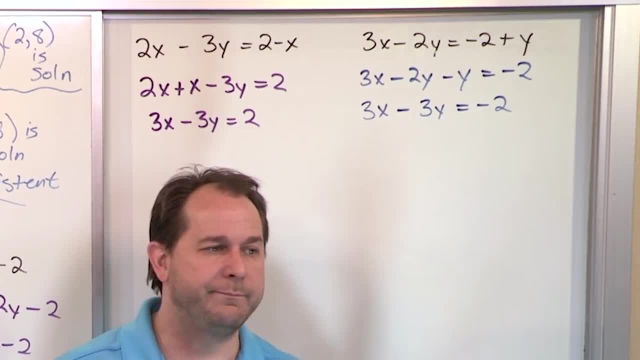 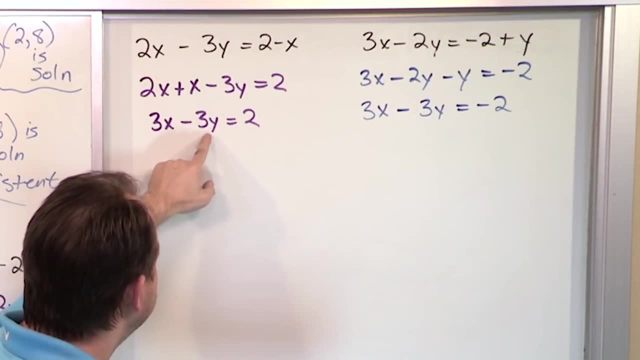 We need to solve for something. in order to solve for something, Okay, We need to substitute it into the other side. You have many, many choices on what to do. I can solve for y, meaning I got to move this thing over here. divide by the negative 3,. 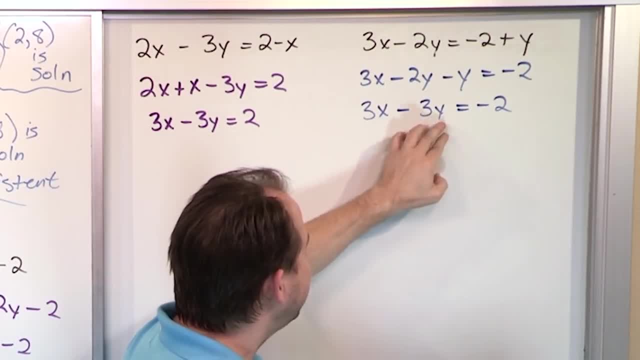 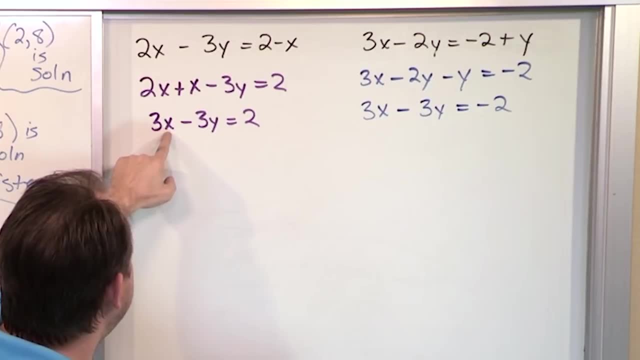 and then when I solve for y, I can stick it into the y value here and then I can find x and I can go on from there. Or I can solve for x. actually, I don't have to always solve for y, I can solve for x, meaning I'll move this over here- divide by 3, I'll have an x value. 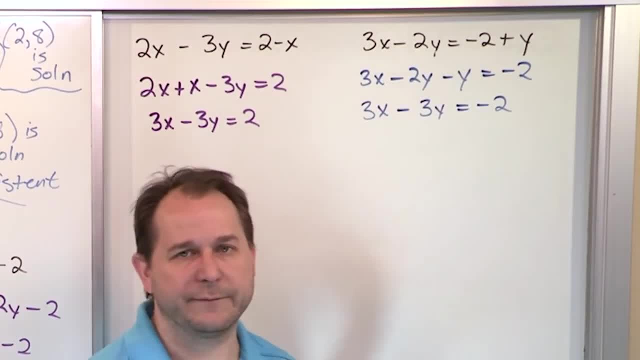 and then I'll stick it into here and then, when I get all the stuff down, I'll be solving for half the solution that way. Okay, That's fine. The only problem- it's not really a problem. I'm trying to teach you different ways to. that's the. that's, of course, fine. 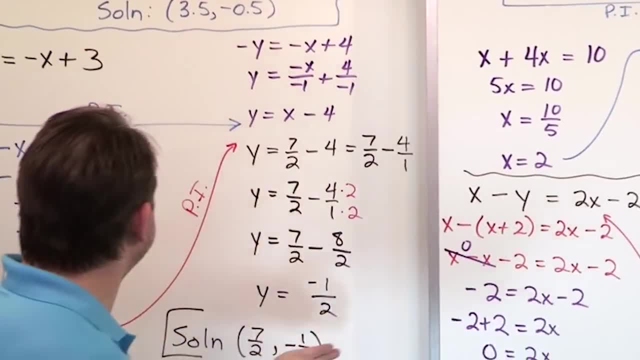 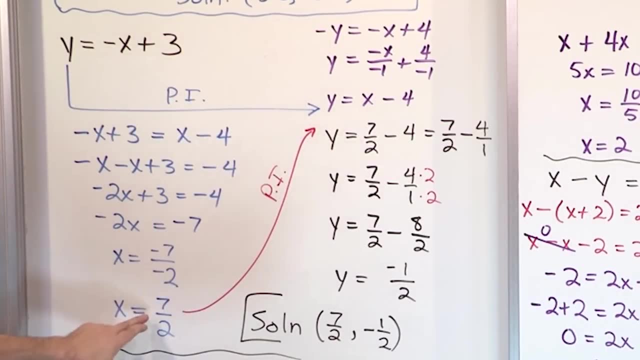 Okay. But you notice what happens sometimes in our very first answer, in our very first problem. Sometimes what happens is when you get down and you do substitutions, you get down to where you have fractions And then you have to plug in a fraction into the other equation and you have to deal with. 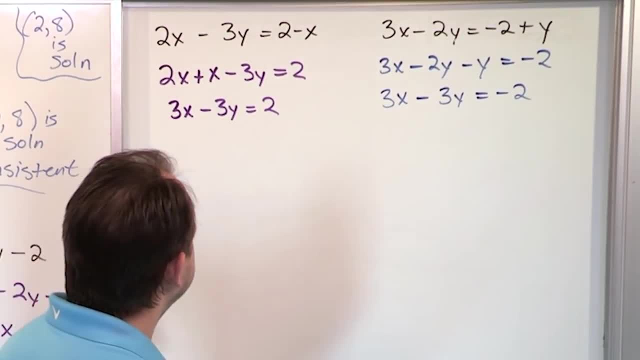 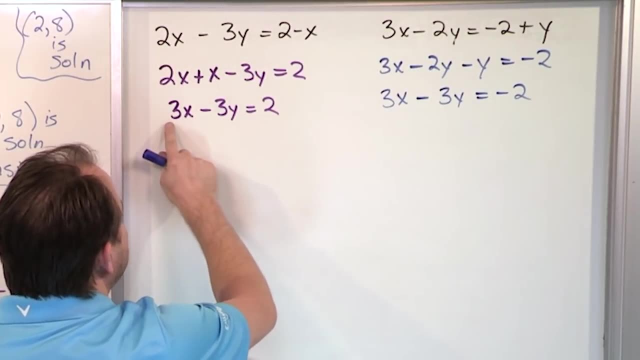 a lot of fractions. Okay, Here I'm in a situation where I have to decide what to substitute in. Okay, So if I solve for x, I'm going to move this over and divide by 3.. I'm going to have a fraction over here somewhere, because 2 divided by 3 is a fraction. 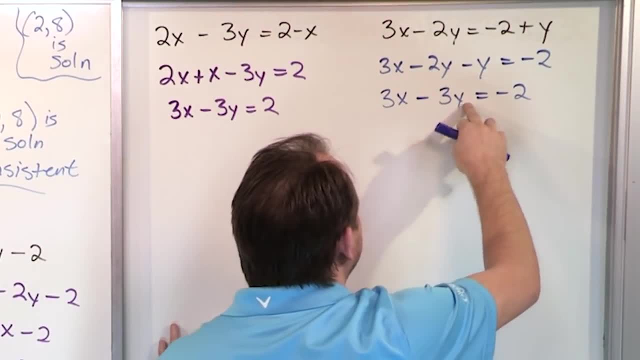 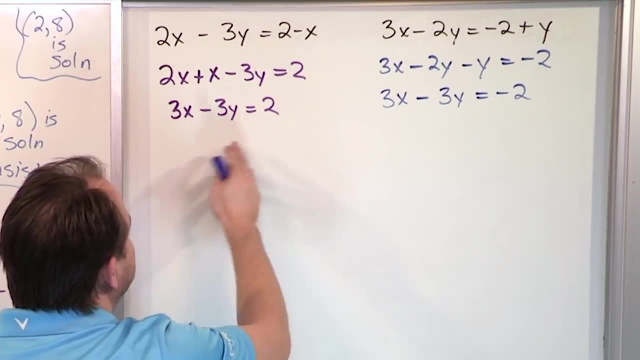 So I'm going to have to. when I plug it in, I'll have to have a fraction inside of whatever I plug in, which means I have a lot of fraction math all right. And if I decide to solve for y, I have the same problem. 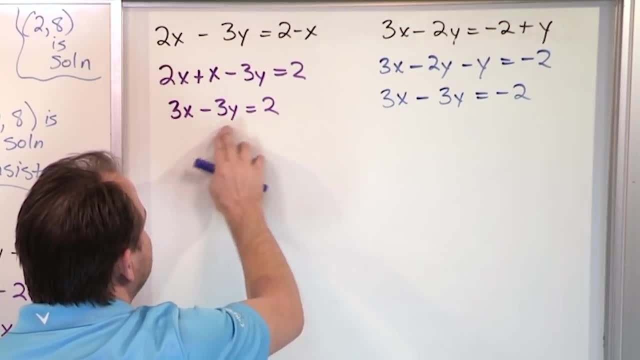 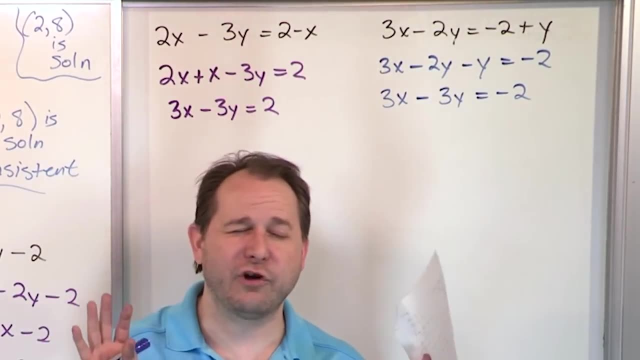 I'll move this over: divide by the negative 3.. I'll still have a fraction, because 2 divided by negative 3 is a fraction. So when I move the y in here, I'll have fractions to deal with. I'll have all kinds of things, which is totally fine. 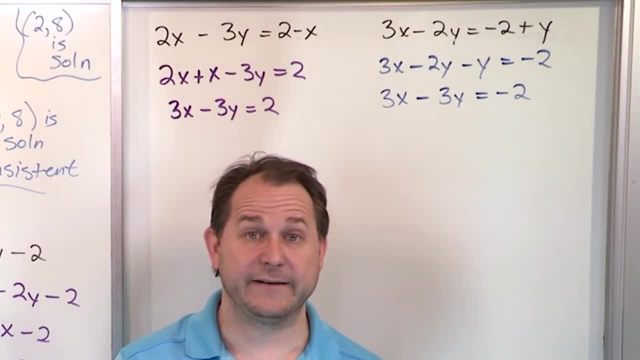 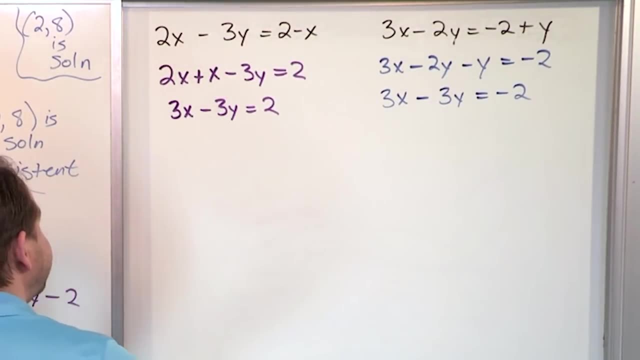 I want you to know how to deal with it with fractions, But in this case there's actually an easier way. So it's not a shortcut, but it's just something that you can notice. Notice that I have a 3x here and I have a 3x here. 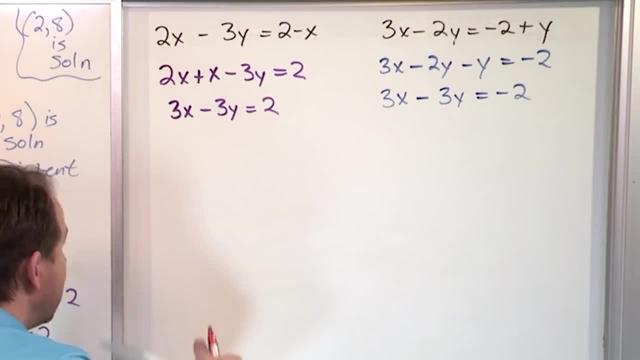 So instead of solving for x and putting x in, let me just solve for 3x. If I just solve for 3x, if I move this to the right, it'll be 3y plus 2.. You understand that. 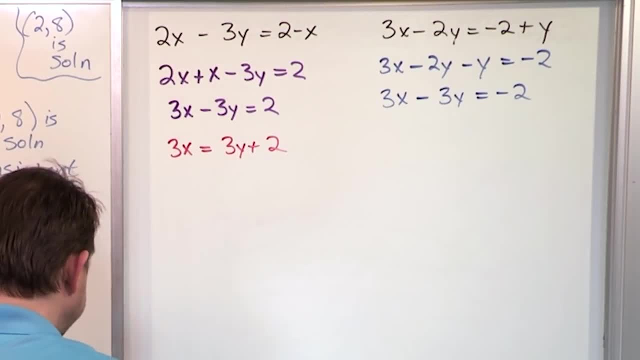 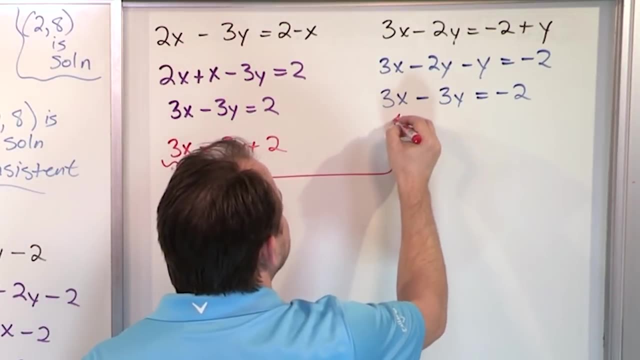 You just add 3y, Add 3y. Now I have this. But you see, it's perfectly fine to take the value of 3 times x and stick it in to here, because I happen to have a value of 3 times x right there. 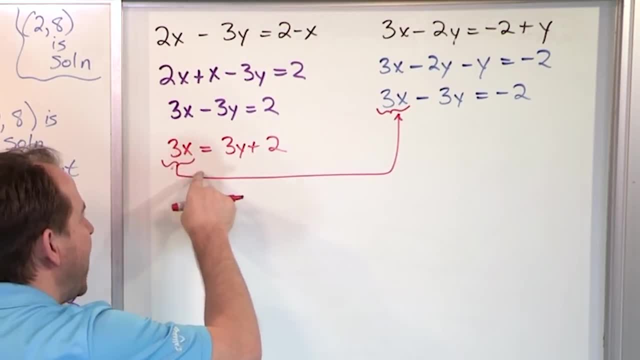 That's perfectly fine. I mean, of course, I could solve for x, meaning I have to divide by 3. See, that's what I'm saying. You'd have the fractions, And then the fractions would have to go in here. 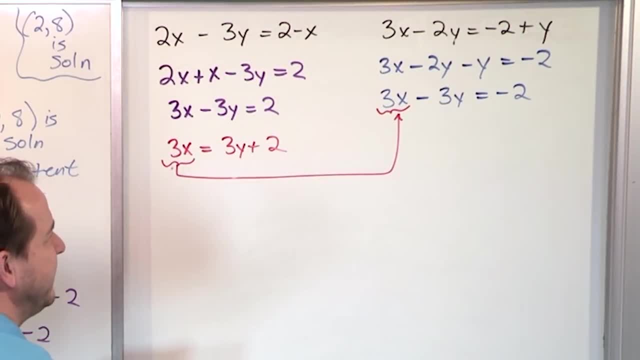 And that's totally fine. It's just you're going to have to deal with all of the fraction arithmetic to get the answer. But in this case there's a 3x here and there's a 3x here. So instead of solving for just x or just y, let me just solve for 3 times x, because remember. 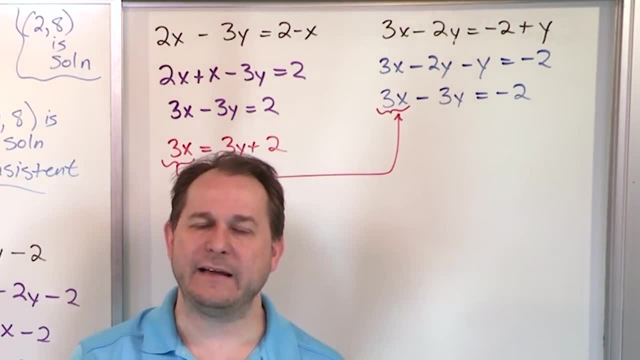 whatever x is, it means I can substitute them in. So that means if I can substitute in for x, then I can also substitute in for whatever 3 times x is. Whatever it is, 3 times x in one equation has to be the same as 3 times x in the other. 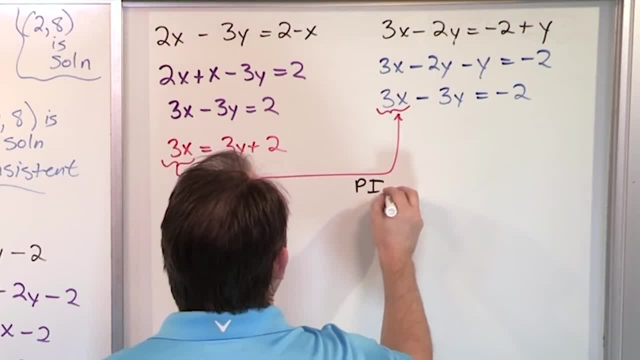 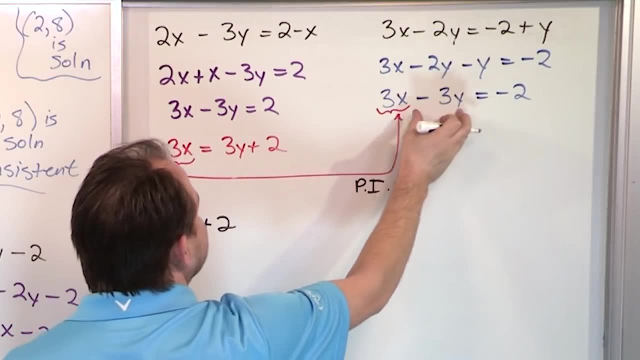 equation. So when I plug in here, what do I get? When I plug in here, I'll have 3y minus 3y. Okay, Minus, I'm sorry, plus 2.. That goes in here. Then I have the minus. 3y is negative 2.. 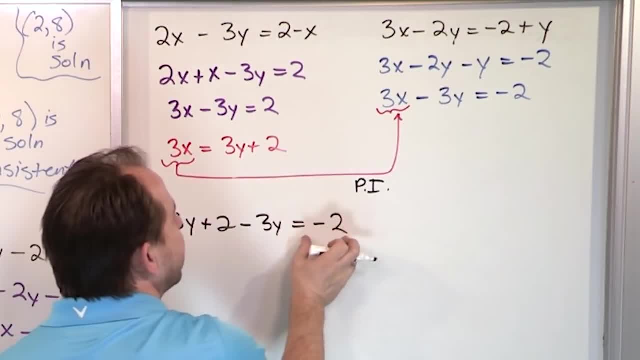 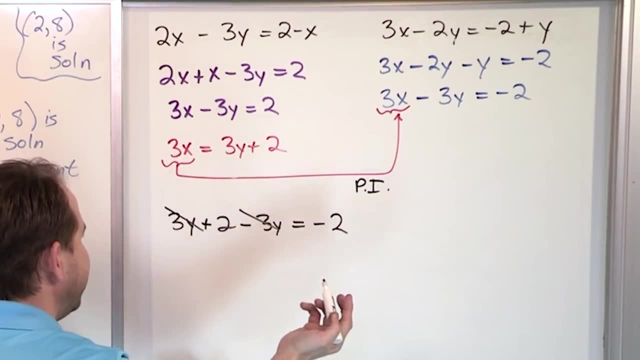 I've just taken this value, I've stuck it in, right there Minus 3y. Here I go. Now what do I get? I have this cancels with this, because 3 minus 3 is 0. So what do I get? 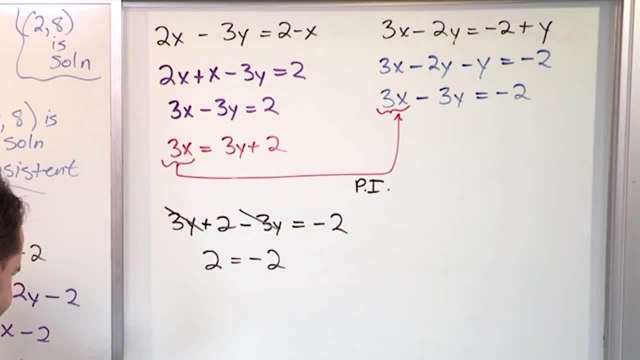 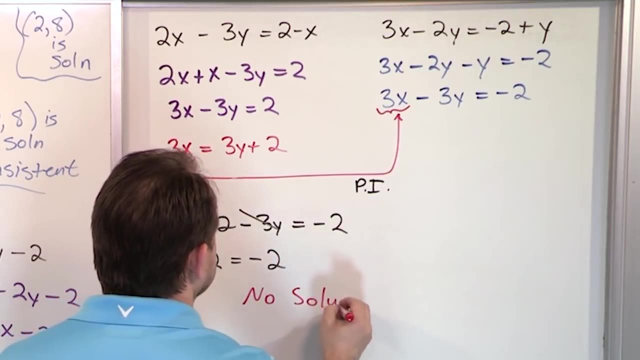 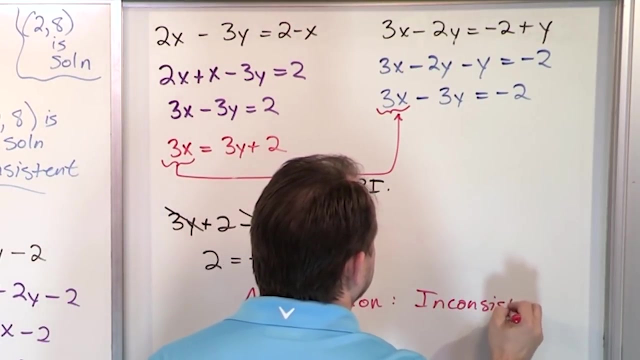 I have 2 on the left, negative 2 on the right. That is impossible. There is no way that 2 can ever be equal to negative 2.. What this is telling you is: it's impossible, So there is no solution, which means they're inconsistent. 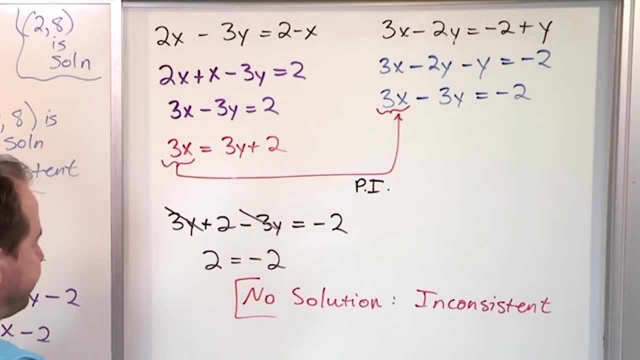 Inconsistent. all right, This is what this is telling you. If you ever substitute in someplace and you start to get a nonsense answer that's never true, that means that it can't be true. What you've put in there is impossible. 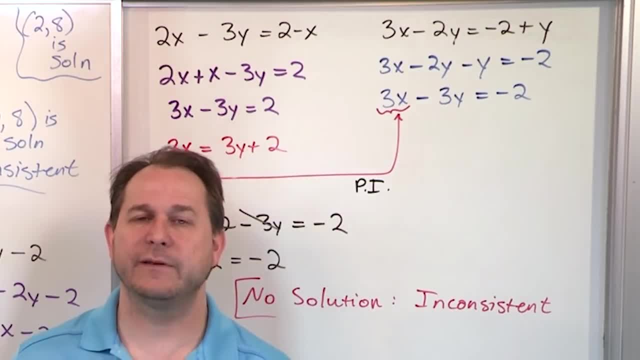 What you've put in there is impossible. What you've put in there is impossible. The x values have to be the same. That's what this is telling you. You put it in there saying, hey, the x values have to be the same at the intersection point. 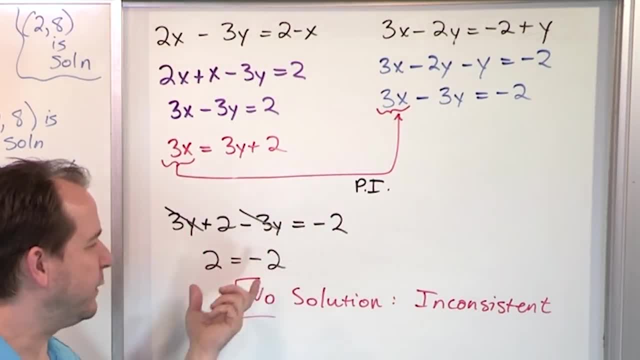 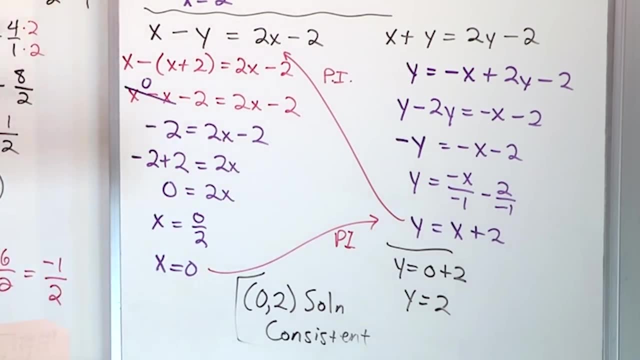 But when I put it in there, I get something completely impossible: That 2 is equal to negative 2 and the variables all drop out At every other problem. when we substituted in, we were able to get an answer. When we substituted in, we were able to get an answer. 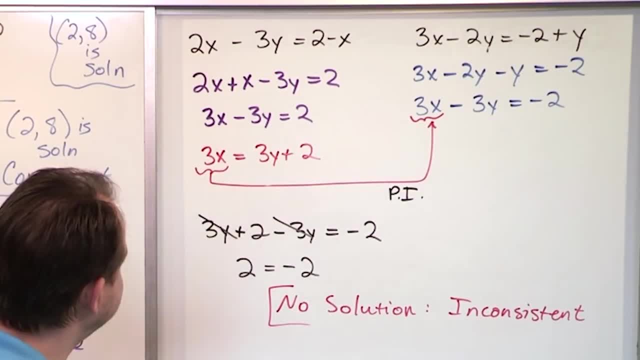 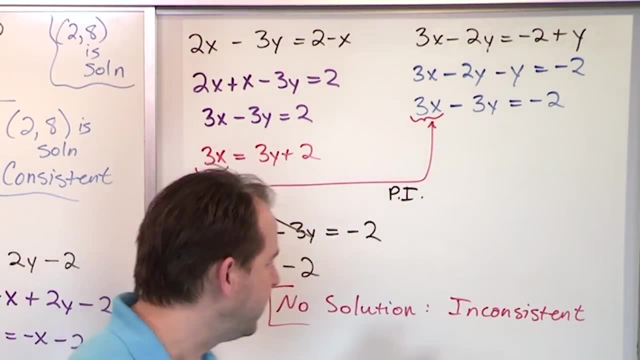 When we substituted in here, we got completely destroyed. We have no way of proceeding. So at that point you stop and you say there's no solution. Inconsistent. How do you know there's no solution? Because this is impossible. You cannot have 2 equal to negative 2.. 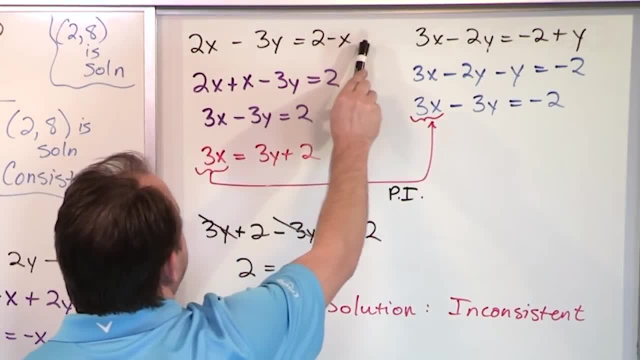 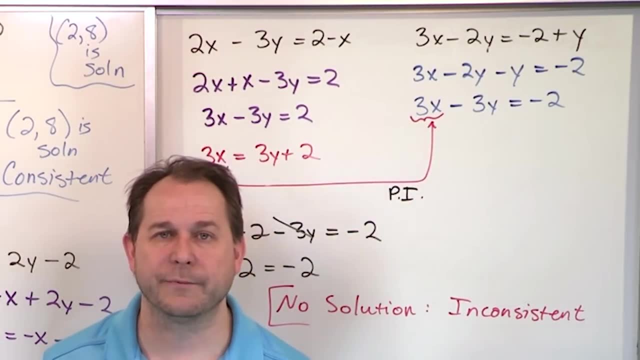 Now, physically, what it means is that if I solve this in mxb plus form, if I rearrange it and I rearrange this in mxb plus form, you're going to find that these two lines have the same slope, They're parallel lines, which means, as we've talked about in the last section, they're